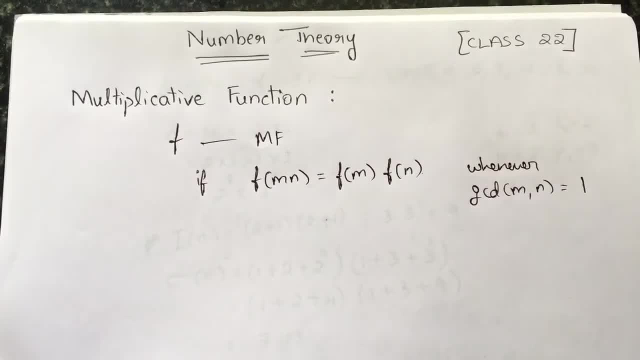 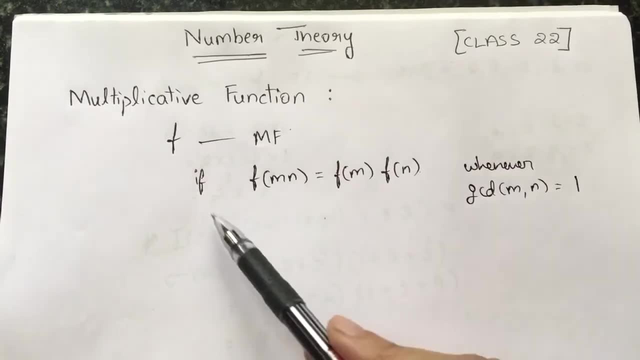 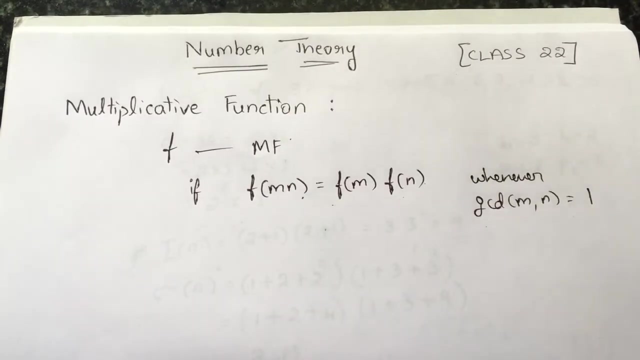 n is equal to f of m into f of n. whenever m and n are relatively prime. Whenever gcd of m comma n is 1. A function number, genetic function, f, is said to be multiplicative function. if f of m- n is equal to f of m into f of n. whenever gcd of m and n is 1., Multiplicative functions arise. 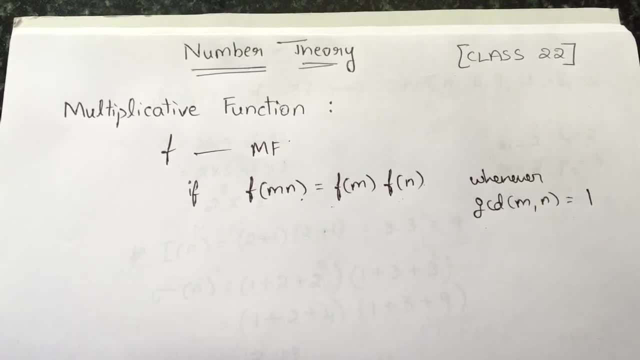 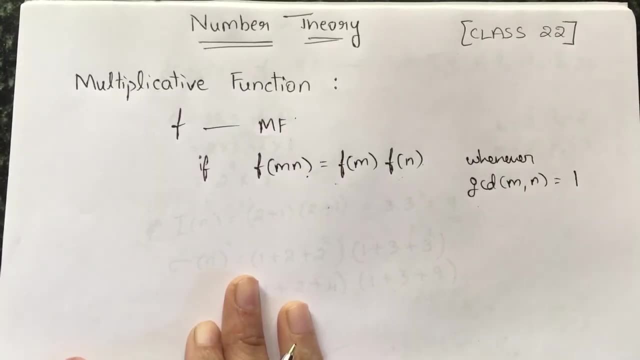 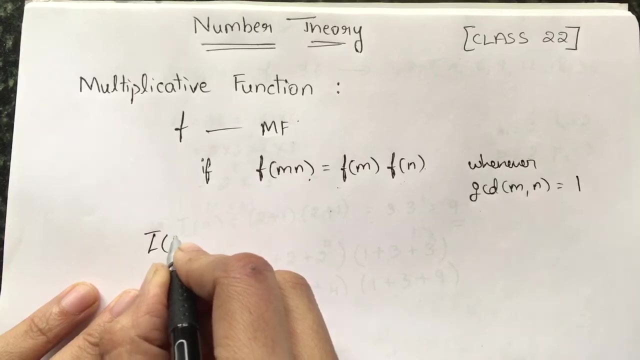 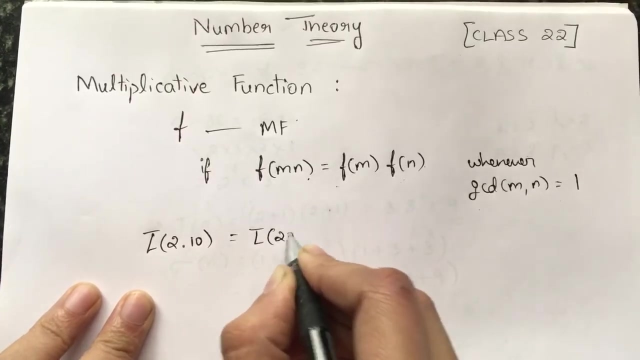 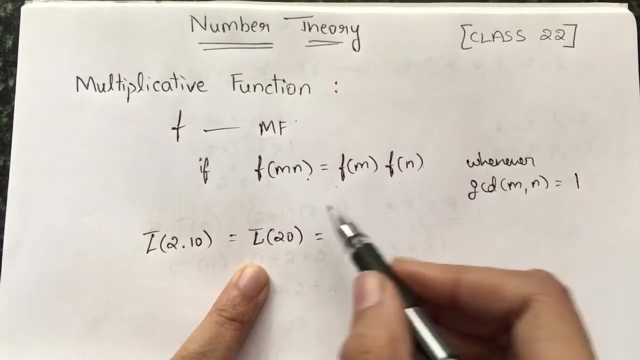 naturally in the study of prime factorization of an integer, When we just observe tau and sigma function. say, suppose I have tau of 2 into 10, okay, tau 20.. How much it is? Tau is nothing but number of positive divisors of 20.. So 1, 2,. 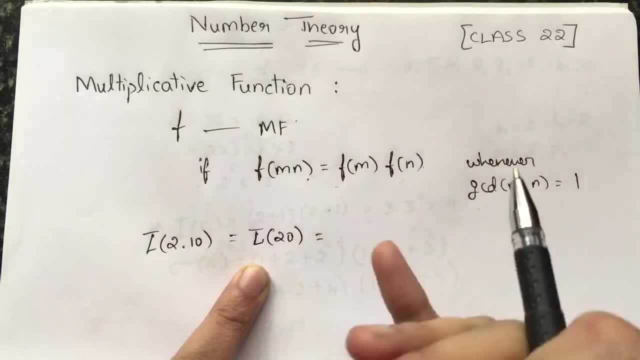 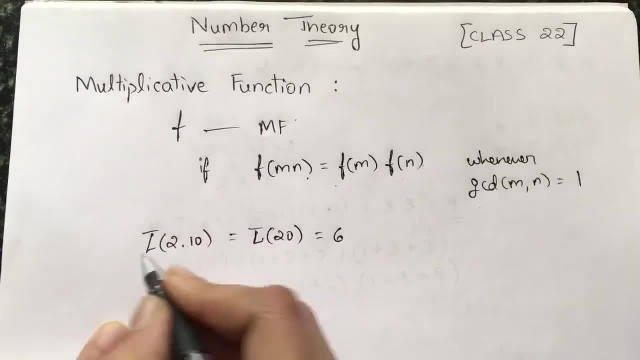 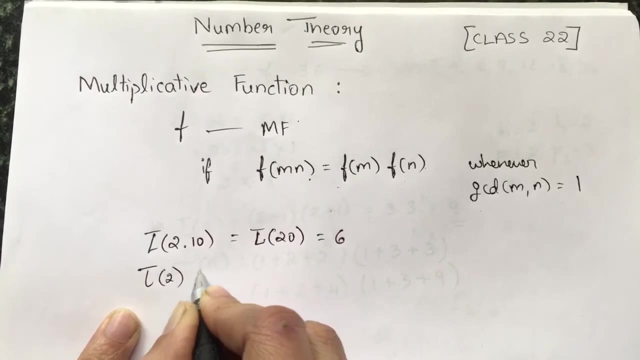 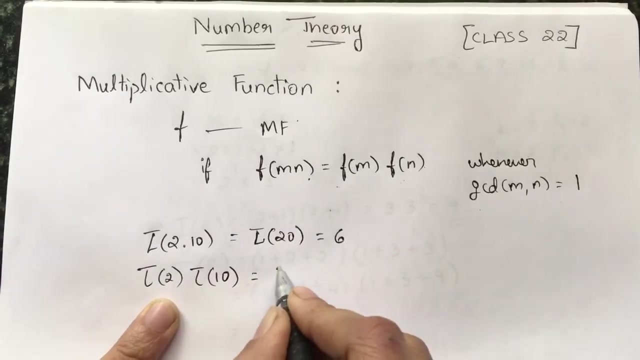 4, 5, and, okay, 5 and 10 and then 20.. So there are 6, right? This I can, if I write it like this: tau of 2 into tau of 10, suppose. Then this is tau of 2 is 2 and tau of 10 is 4, which is equal to 8.. 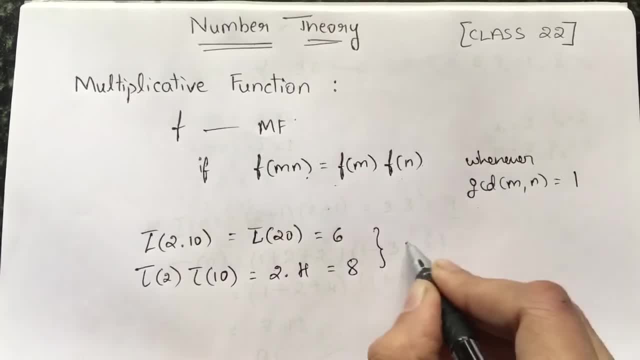 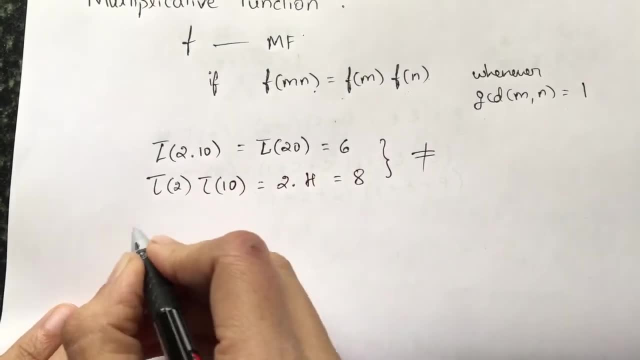 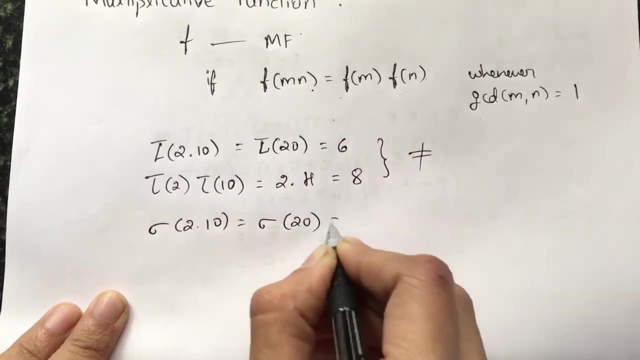 Right. So you cannot absorb that these 2 are not equal right. At the same time, if I take sigma of 20, sigma of 2 into 10, that is sigma of 20, sum of the divisors of 20.. 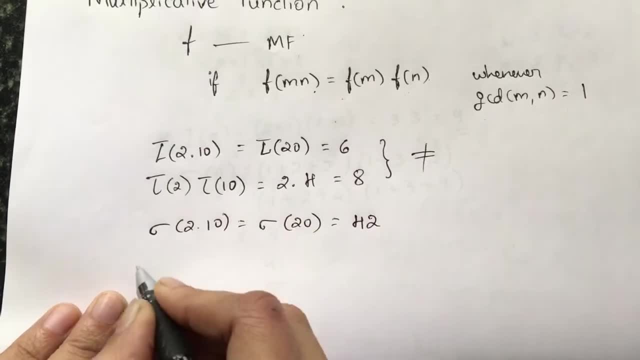 So it comes out to be 42.. And sigma of 2 into sigma of 10, does not mean number of divisors of 10, is equal to 5 and therefore the sum of all the divisors is equal to 0. Themutual suffix. delta gamma for delta C is defined as minus 1 and 넣고. So it is the means right Now. if you take, if I take, sigma of 20 in to 10, that is sigma of 20, then drops across at here. and then there are 4. container numbers. So here I have two, two, two of 2, plus m�, and what is it? So? y plus alpha, N and CA, so it takes 1 to patients of middle of the. 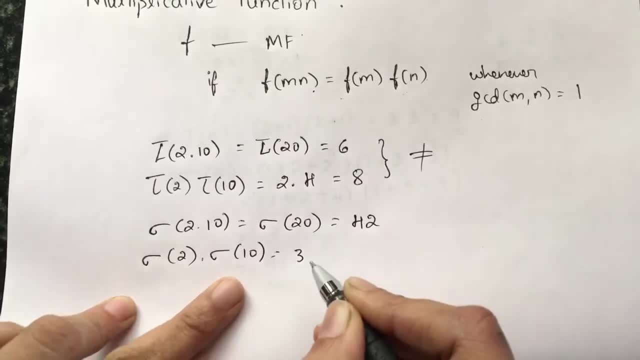 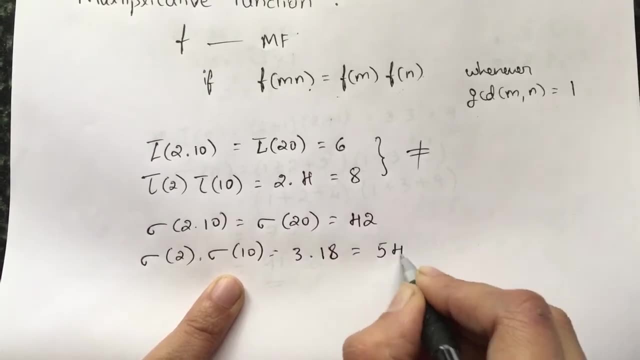 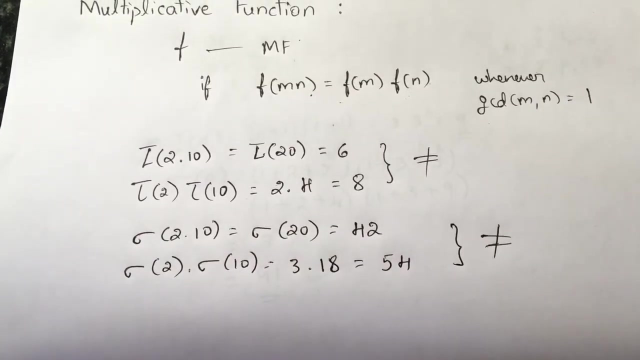 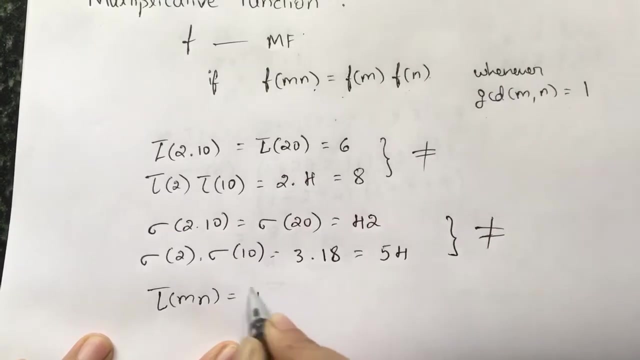 sigma of 2 is 3, 2 plus 1, and sigma of 10 is comes out to be 18, so 54, and they are not equal right. so it is need not be true that tau of m? n, tau of m? n, is equal to tau of m. 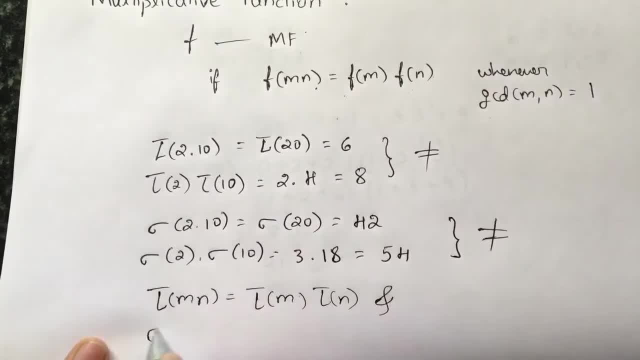 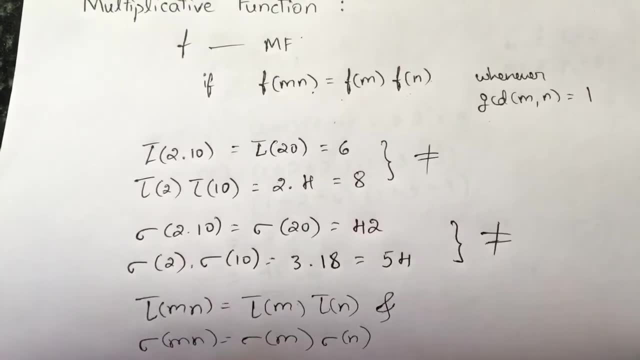 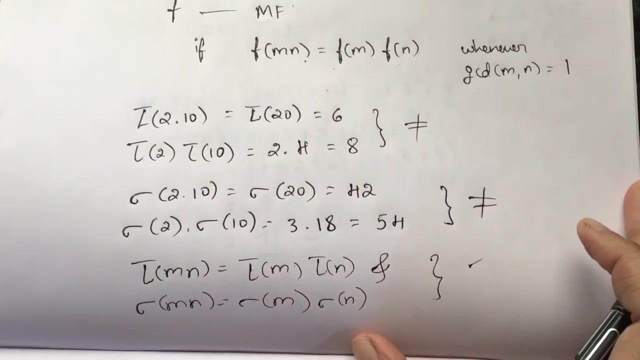 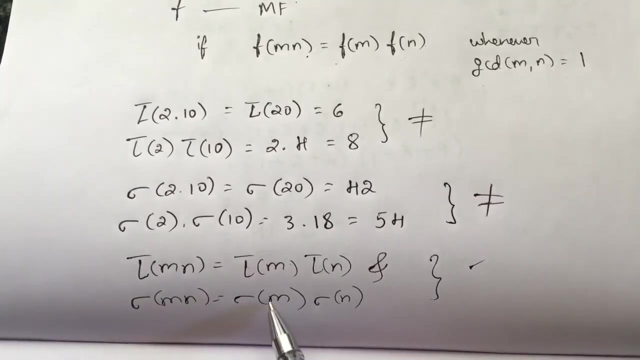 into tau of n and sigma m n is equal to sigma m into sigma n. this means it is not necessary that they have to be equal right equality always holds, provided we stick to the prime numbers m and n. if m and n are prime in the sense they are railing. 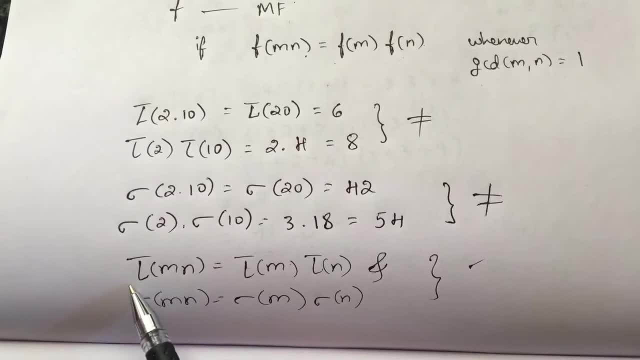 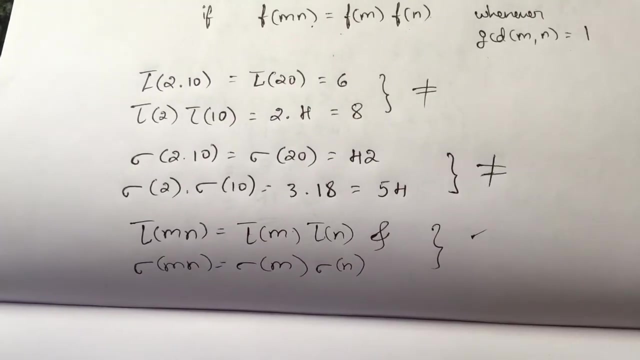 relatively prime, then we can say that tau of m? n is equal to tau m into tau n and sigma m n equal to sigma m into sigma n. If gcd of m? n is equal to 1,, then f m n equal to f of m into f of. 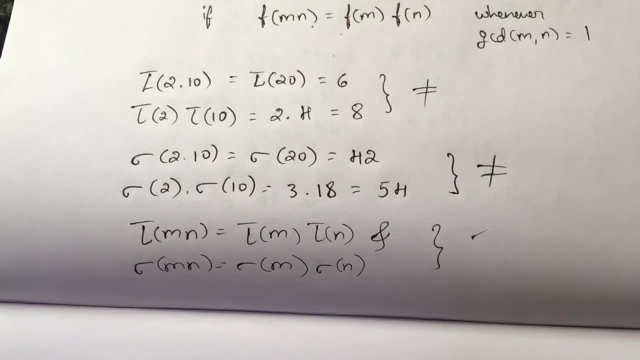 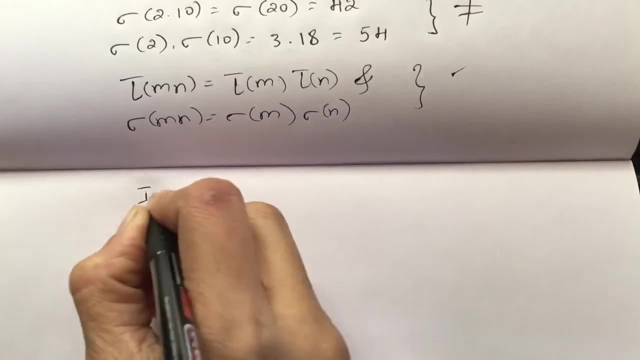 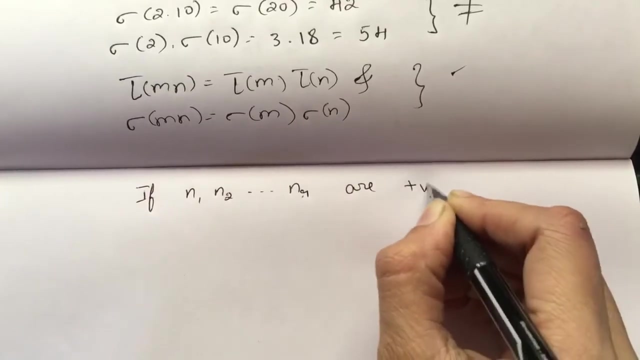 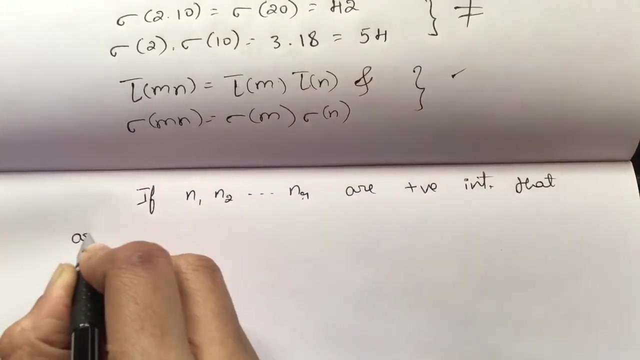 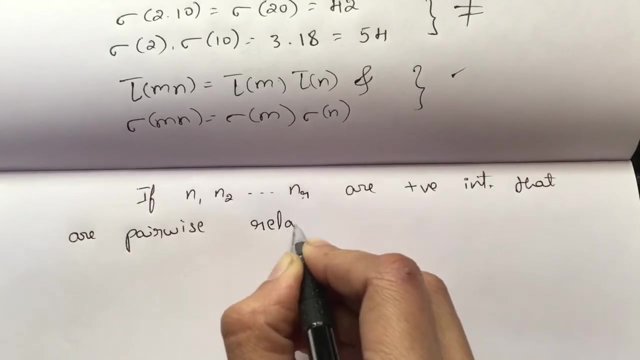 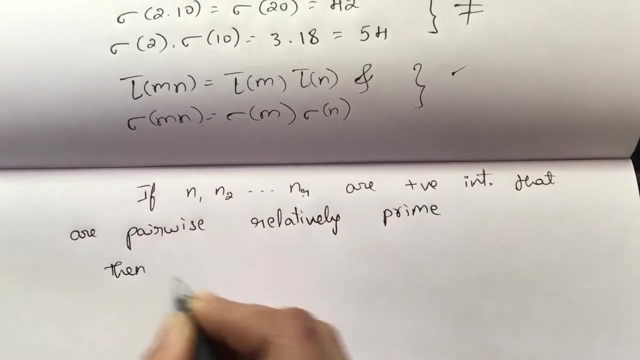 n means f is a multiplicative function. okay, If suppose, if n1, n2 dash, dash n are positive integers, positive integers that are pairwise primes, pairwise relative, Relatively primes- I mean to say relatively prime- then we can write f of n1 into n2 dash. 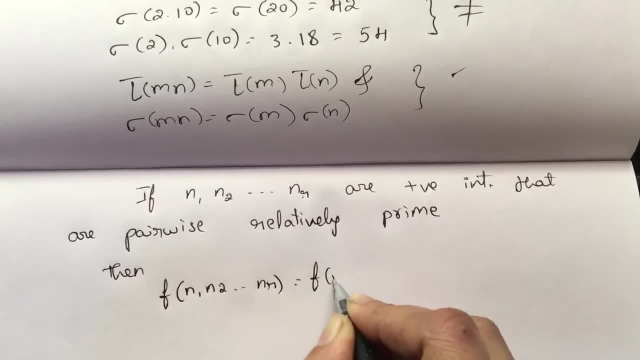 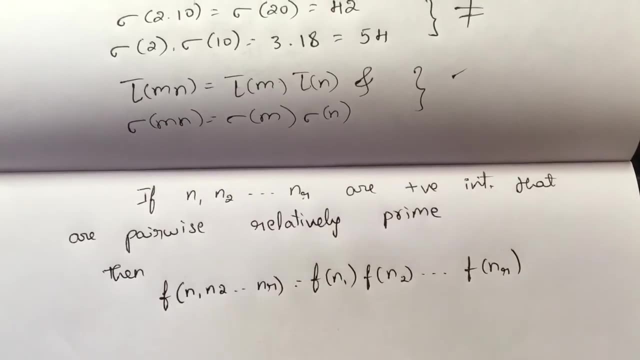 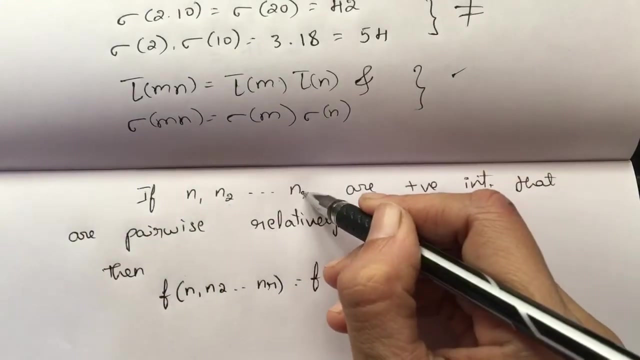 dash n are equal to f of n1 into f of n2 up to f of n are okay If n1, n2, n3 dash dash n are relatively prime in the positive integer, which are pairwise relatively prime If that is the 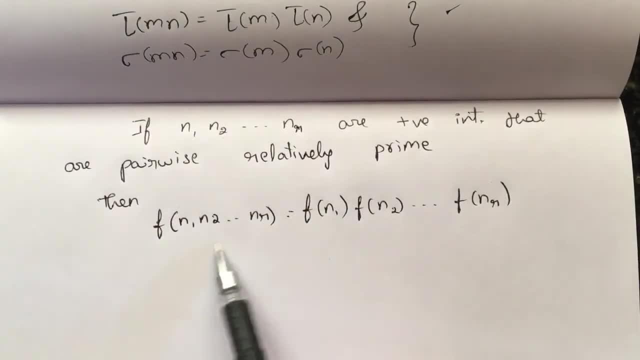 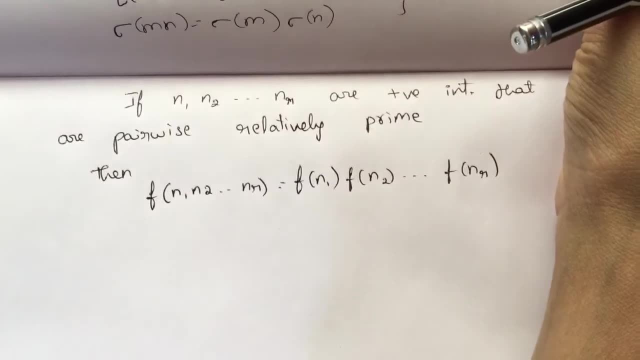 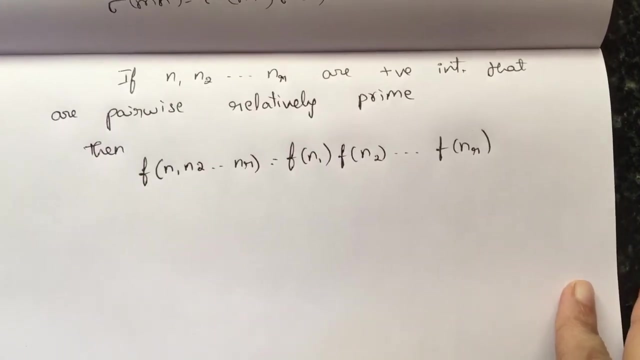 case, then f can be written like this, so that f is a multiplicative function. The big advantage of this multiplicative function is they are completely determined once their values at the prime powers are known to us. Suppose n is greater than 1,. 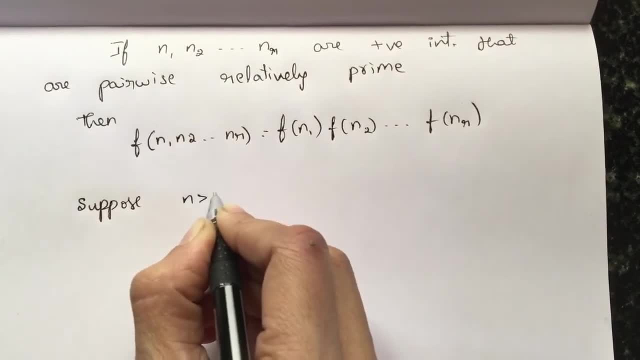 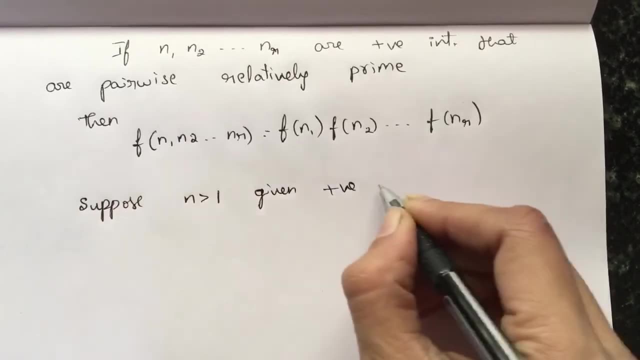 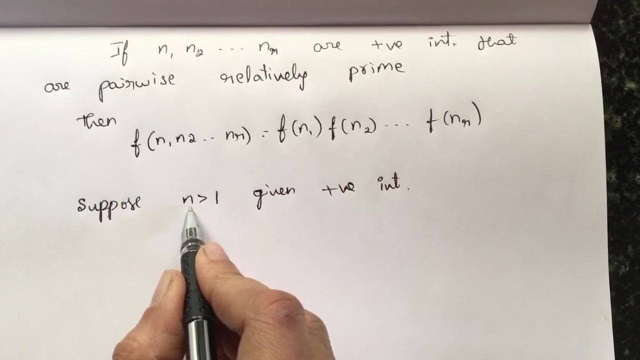 n is greater than 1, this value is given to us. okay, It is a given, in fact a positive integer. Then we can write the canonical form of n. that means I can write n as product of primes right. n can be written as product of primes p1, power, k1,. 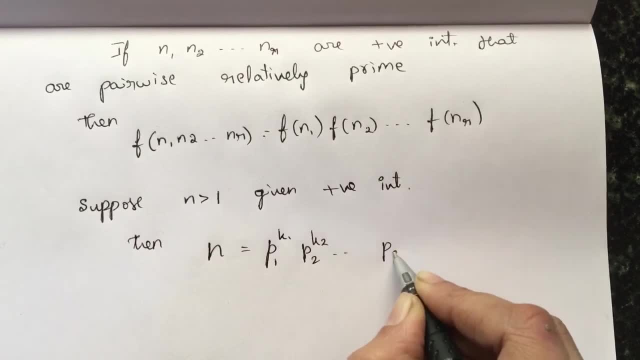 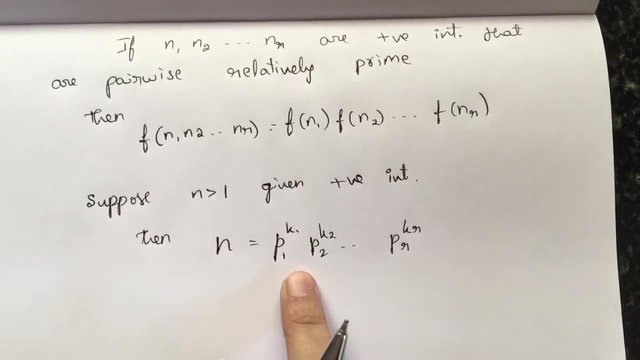 p2 power k2 into, say, pr power kr. Since these pi power ki are pairwise relatively prime, in the sense when you take a pair of pis they are relatively prime, then we can write f of n as f of p1 power k1.. 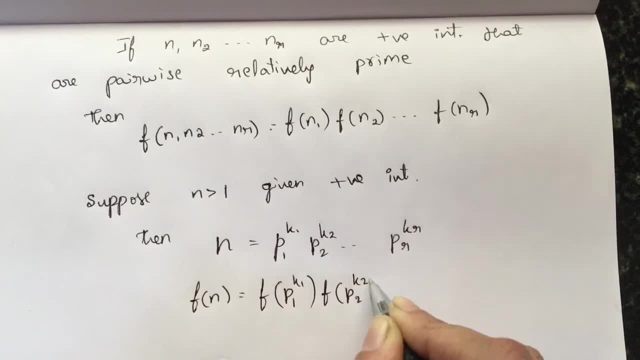 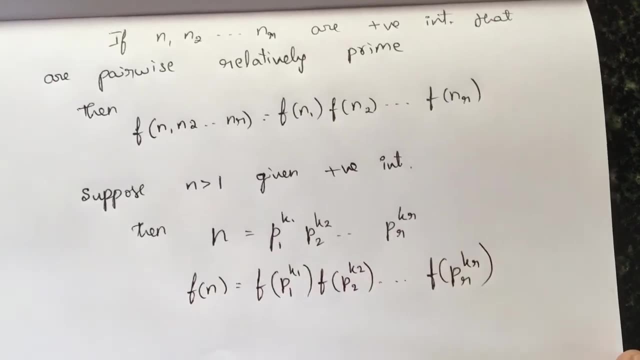 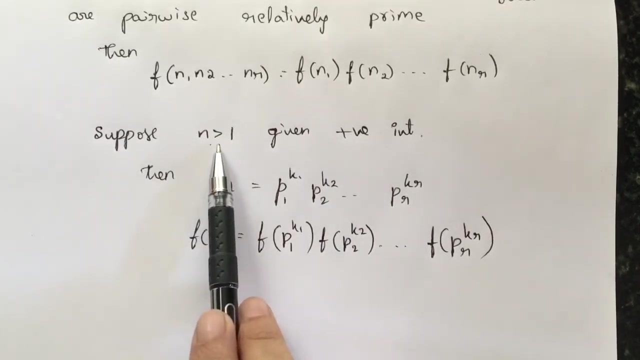 into f of p2 power k2, like that f of pr power kr. okay, This is possible when pis are relatively primes. Here, say, I have mentioned n as a positive integer greater than 1, so it can be written in: 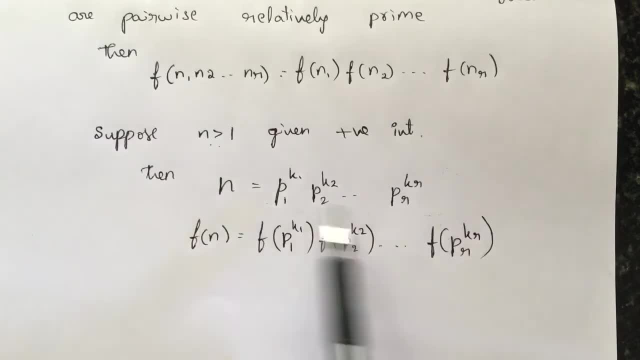 terms of product of primes. that means a canonical form of n. So when this is written, f of n can be written like this: So this is the canonical form of n. so when this is written, f of n can be written like this: 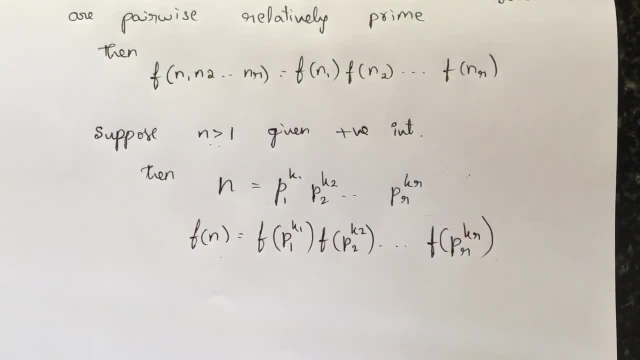 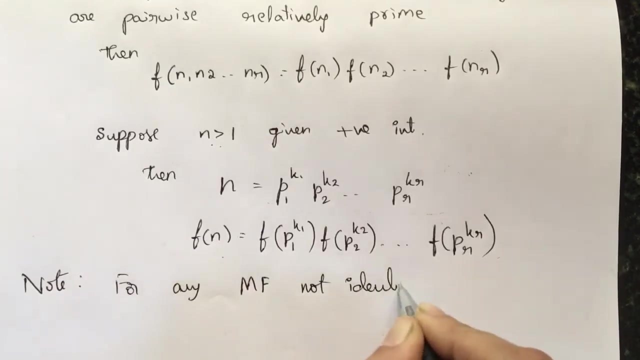 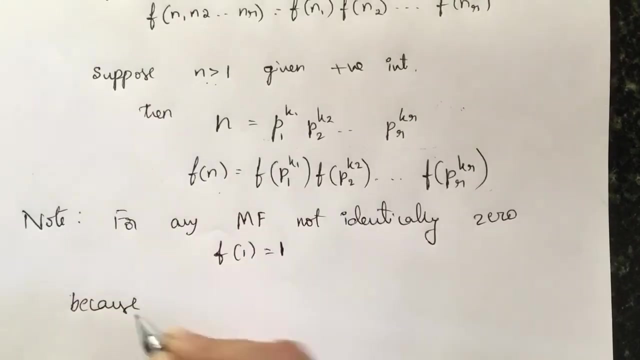 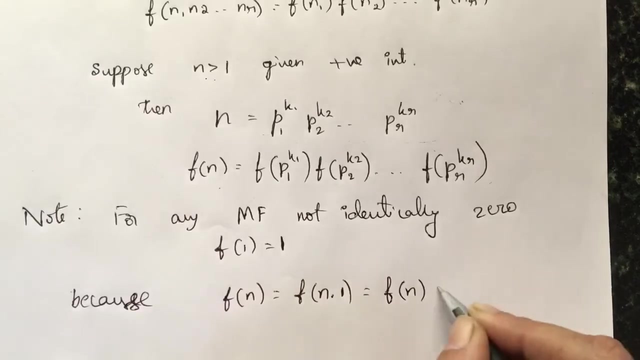 You know one thing: for any multiplicative function not identically zero multiplicative function identically zero, okay, f of 1 is 1.. So this is how- because we can check it out- f of n can be written as f of n into 1, since f is a multiplicative function, this can be rewritten as f of n into f of 1, right? 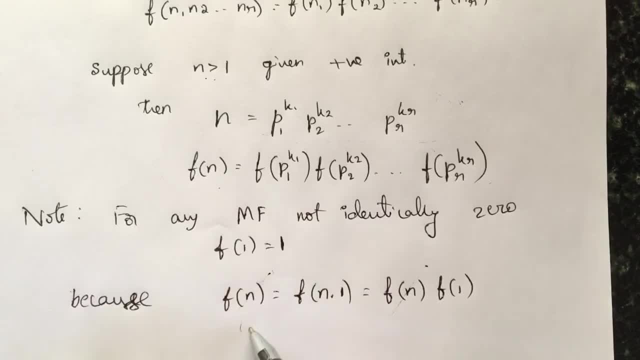 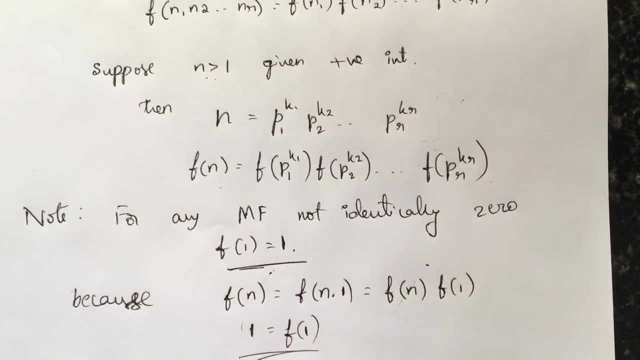 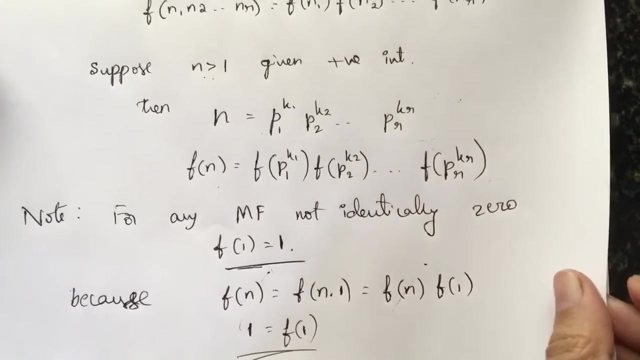 Now if we cancel f of n, both the side, I am getting 1 equal to f of 1, in the sense f of 1 equal to 1.. So for any multiplicative function which are not identically zero, f of 1 is 1.. Now let us prove tau and sigma functions are multiplicative functions. 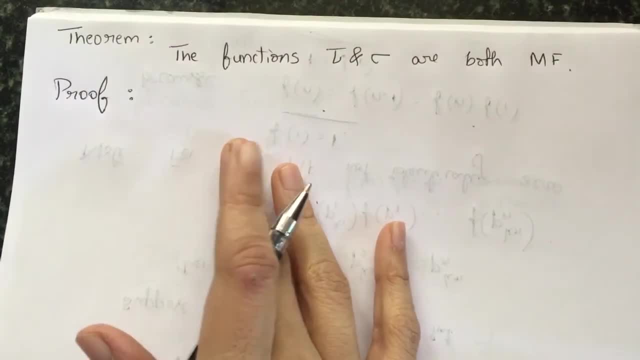 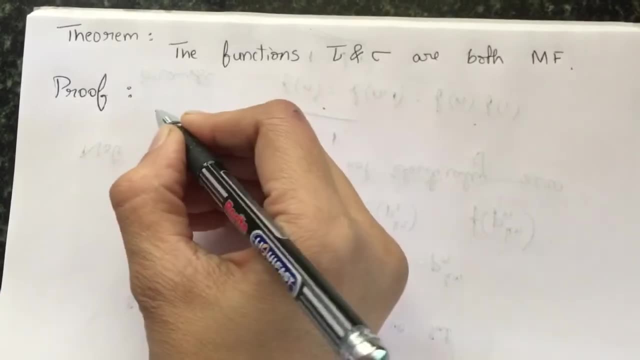 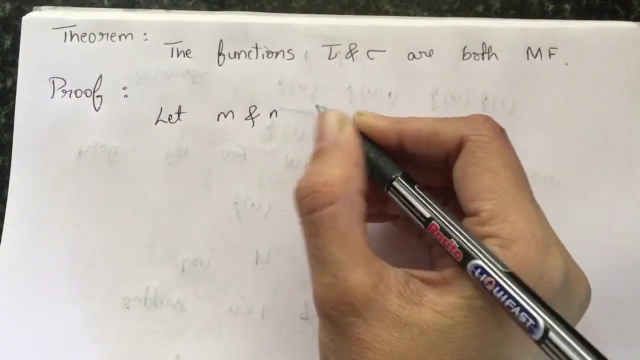 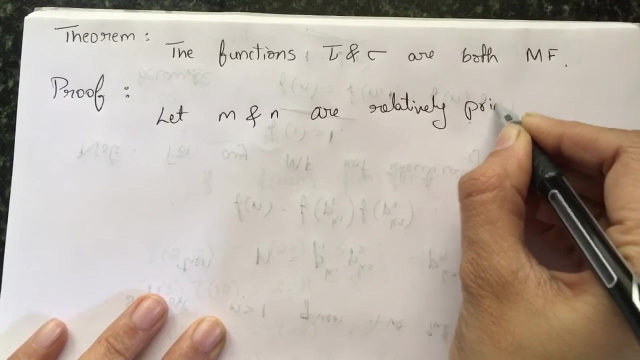 Tau and sigma. both are multiplicative functions. So to prove this, even any one of m and n, suppose I have two numbers, M and N, which are relatively prime, okay, in the sense that GCD is 1. now, among this M and 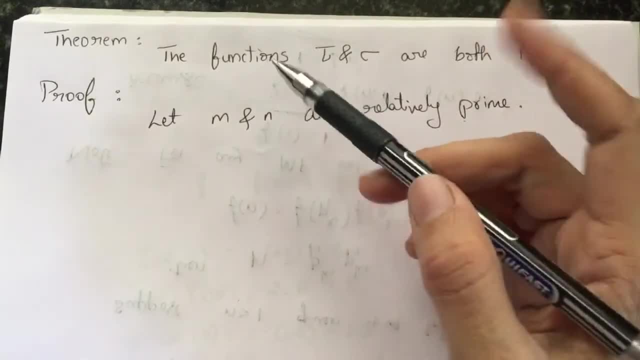 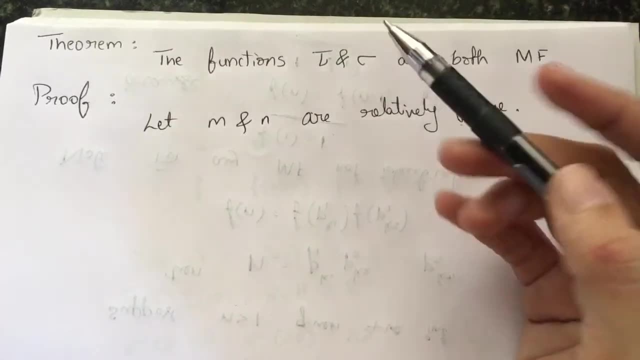 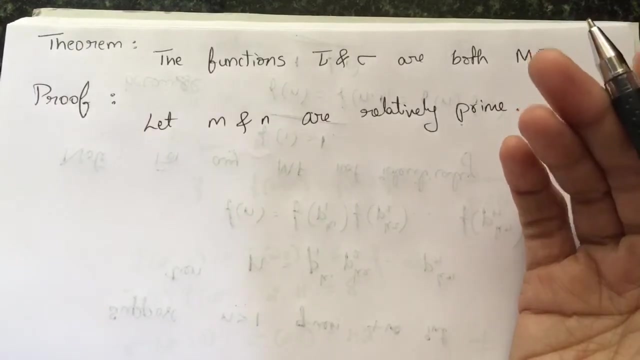 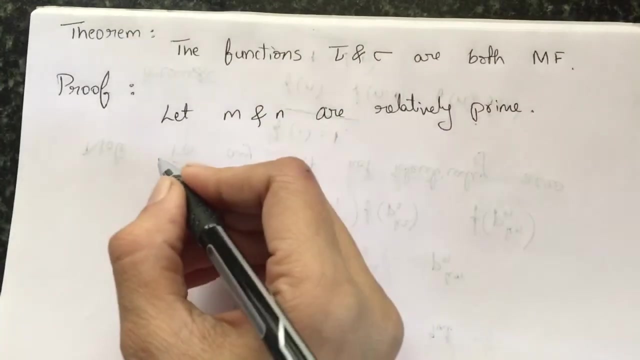 N if any 1 is 1. if any 1 is equal to 1, then the situation is a trivial situation, right? so we are taking M and N which is greater than 1, so the result is true if either M or N is equal to 1. okay, so I am just leaving that. I am assuming that M is greater than. 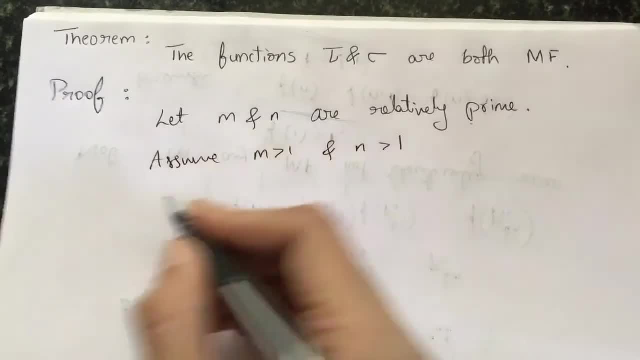 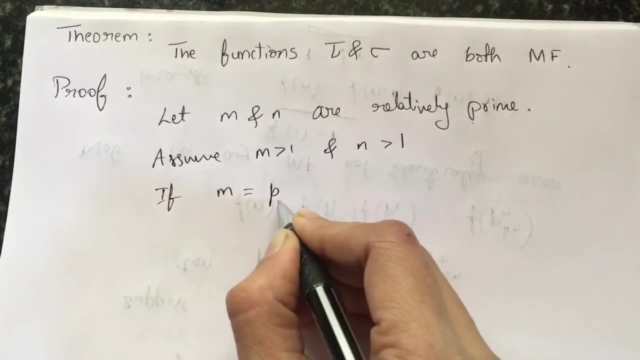 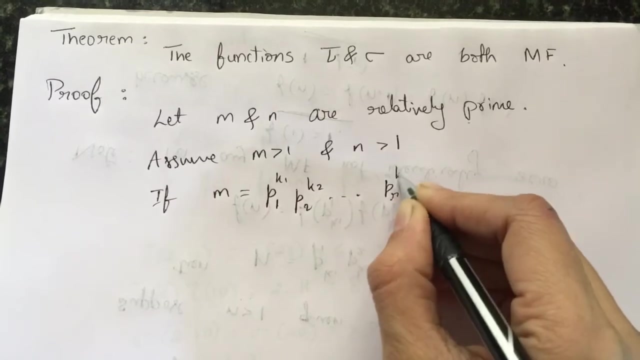 1 and N is greater than 1. okay, and if I write M in its canonical form like this: M and N are equal to 1. so I am assuming that M and N are equal to 1. okay, so I am assuming that M and N are equal to 1. say P1, power K1, P2, power K2 into PR, power KR, and I will. 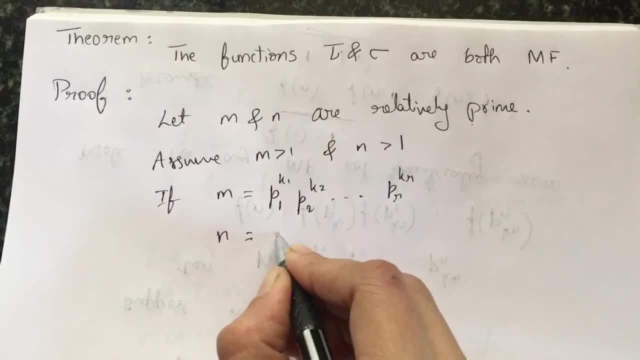 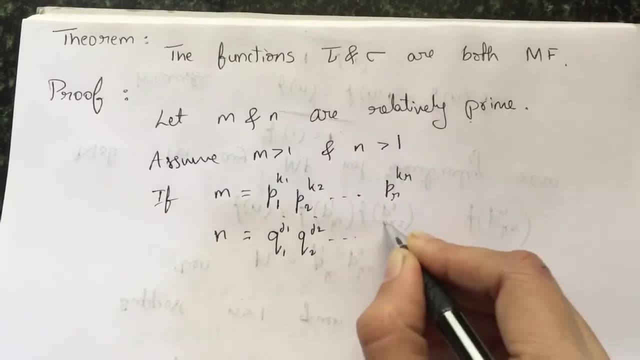 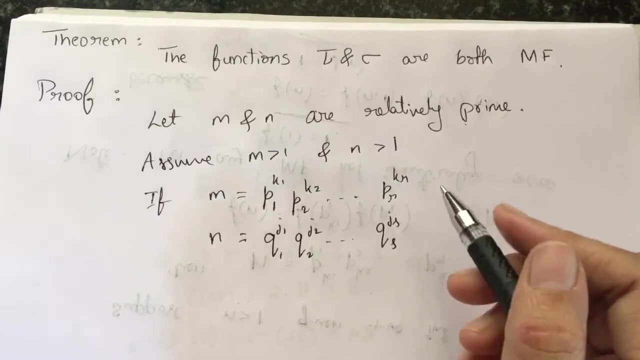 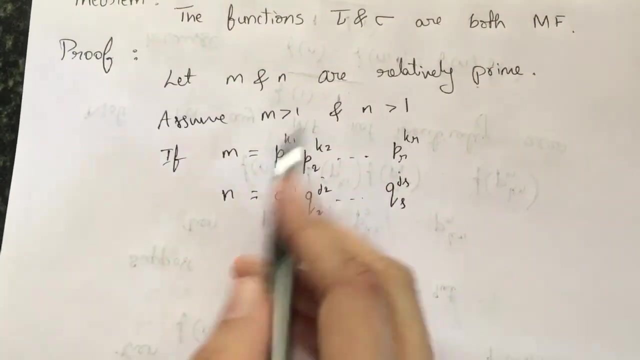 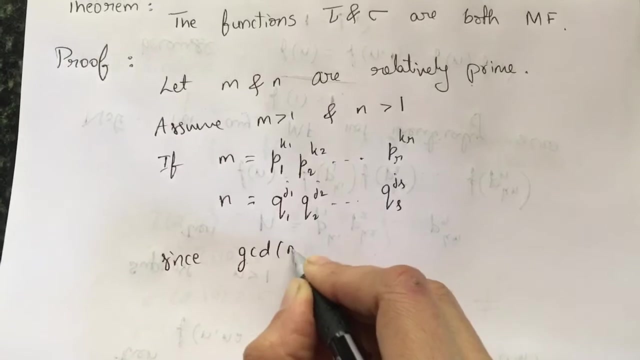 write N as say Q1 power J1, Q2 power J2, like that Qs power Js. these are the prime numbers. okay, factorization of M and N. since it's mentioned that GCD, I'm considering M and N- are relatively prime. therefore that GCD is equal to 1, no PI can occur among. 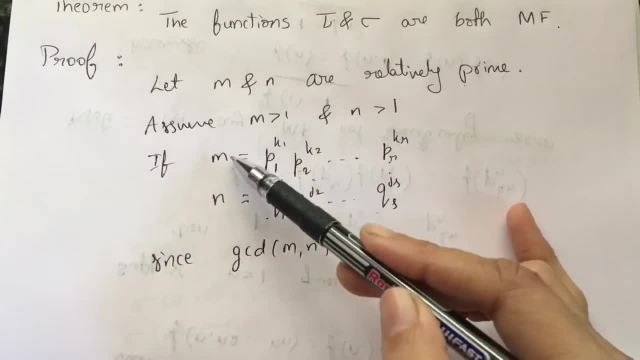 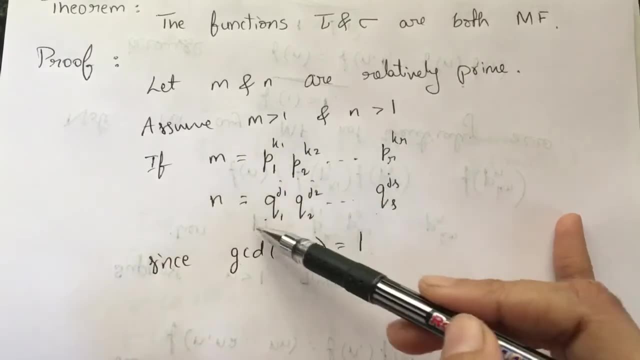 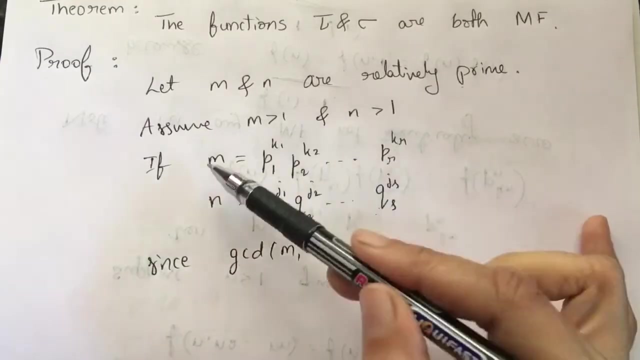 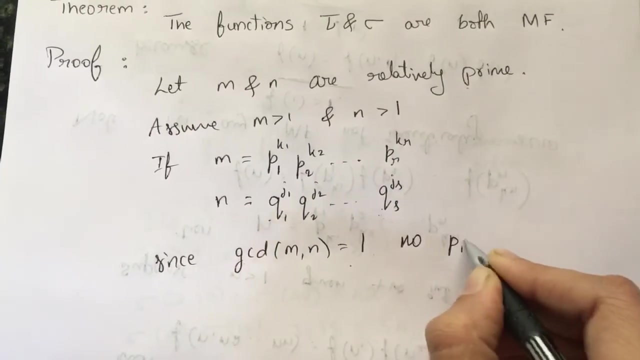 this QJ right, because there is no common factor other than 1 for M and N. therefore, no PI occurs in the prime factorization of N, or no QI occurs in the prime factorization of M. okay, so since their GCD is 1, no PI can occur. 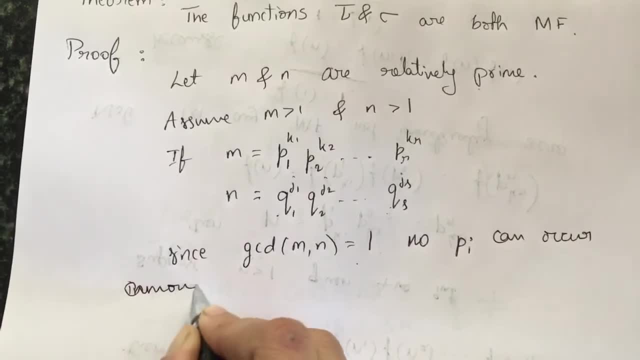 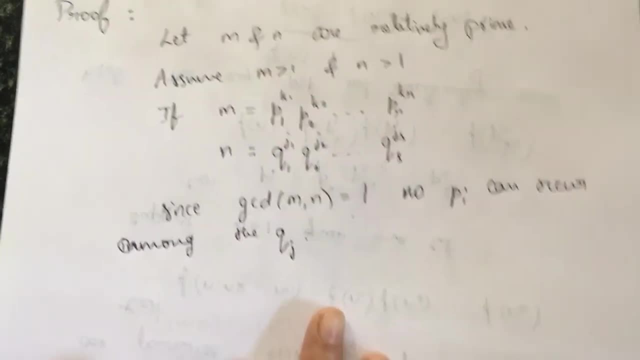 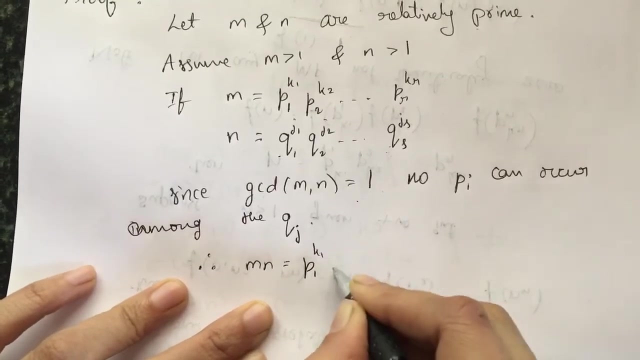 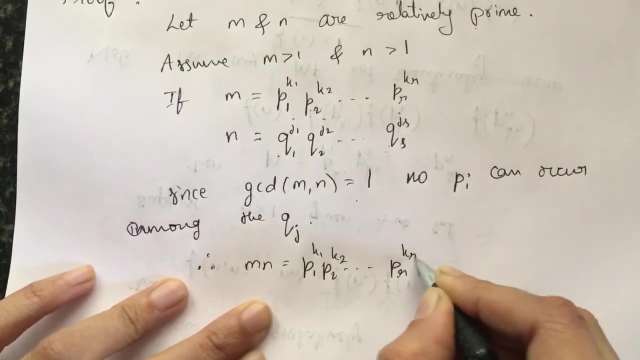 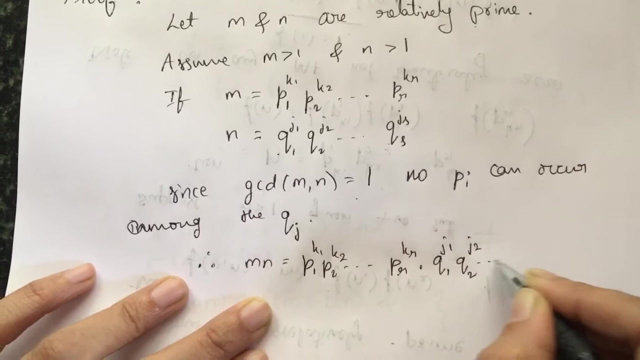 among QJ's. okay, therefore, I can write the product MN M into N, equal to P1 power. K1 into P2 power K2, dash dash into PR power, KR into Q1 power, J1 into Q2 power J2, all the way up to QS, to the power J2. 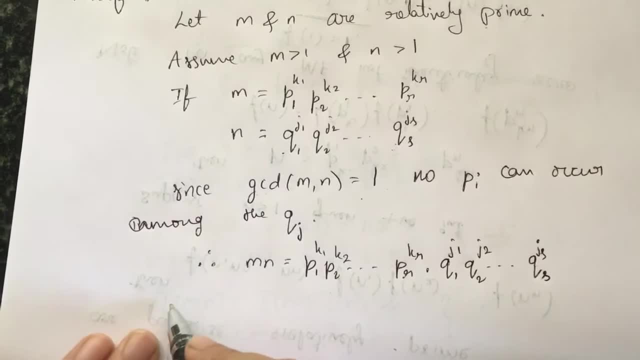 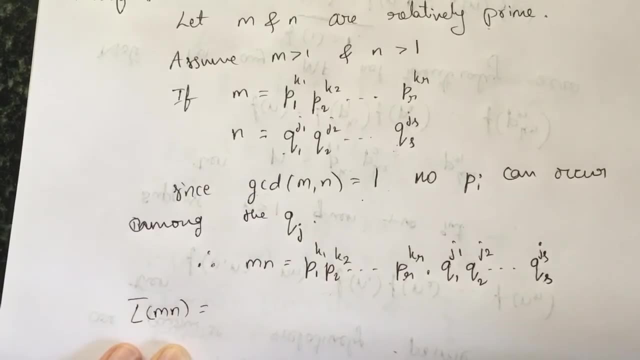 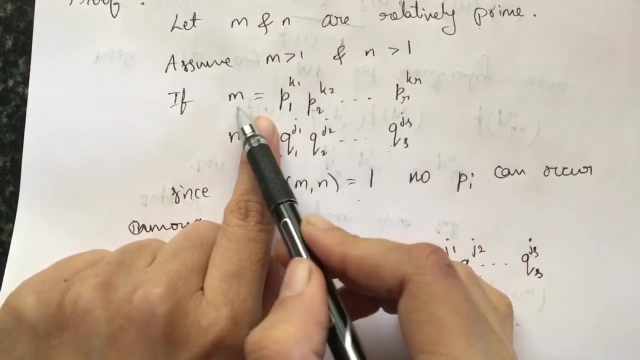 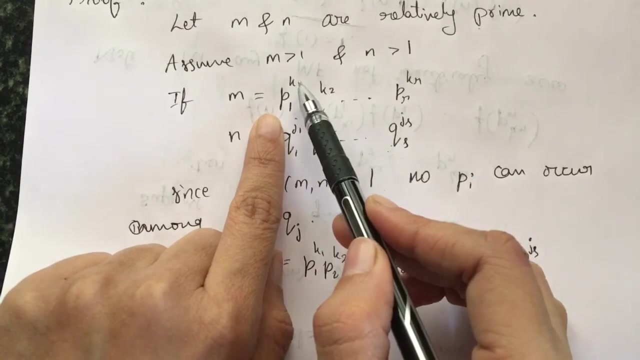 S. okay now. toe of MN M into N equal to C. this is from the formula we know. if M is returned like this, it has got a prime factorization like this. then we know the formula: toe of M equal to K 1 plus 1 into K 2 plus 1, all the way up to Kr plus 1. that we know it has got a prime factorization like this. then we know the formula: toe of M equal to k1 plus 1 into k2 plus 1, all the way up to kr plus 1. that way, knowing means that we have the formula so far. I hope you have an experience following this and I hope this of you also been helpful. learning K6 puzzle. 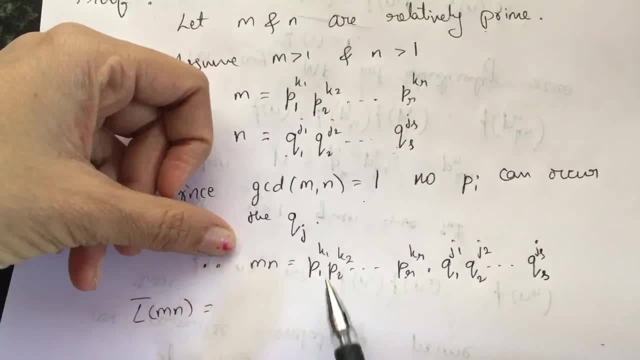 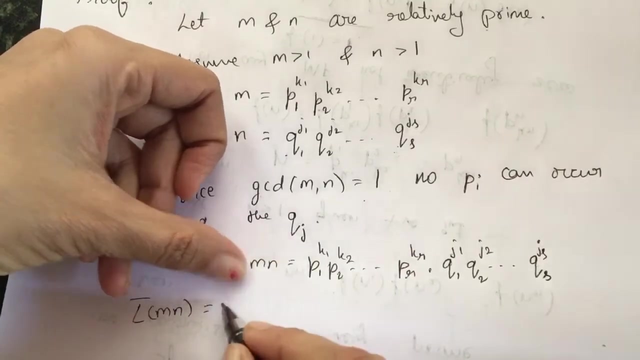 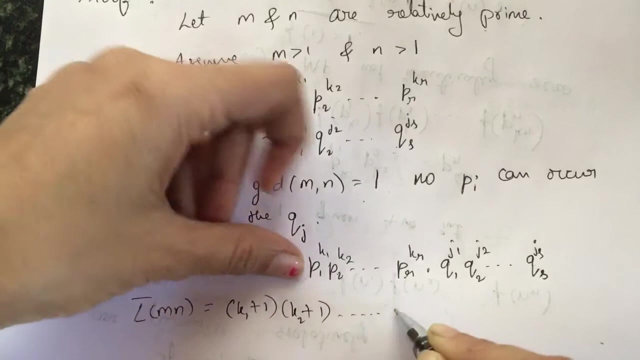 Now here I have written Mn as P1 power K1, P2 power K2 into Pr power Kr, into Q1 power J1, like that till Qs power Js. So tau of Mn is equal to K1 plus 1 into K2 plus 1 up to Kr power, sorry, Kr. 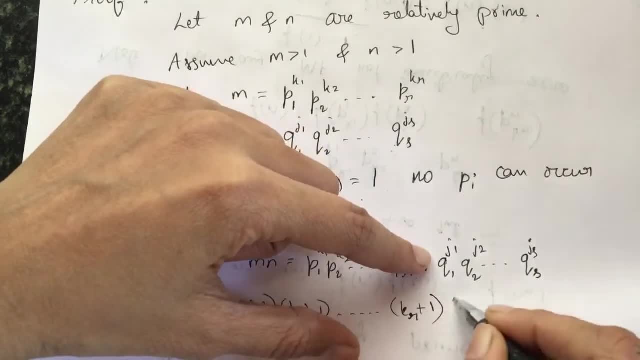 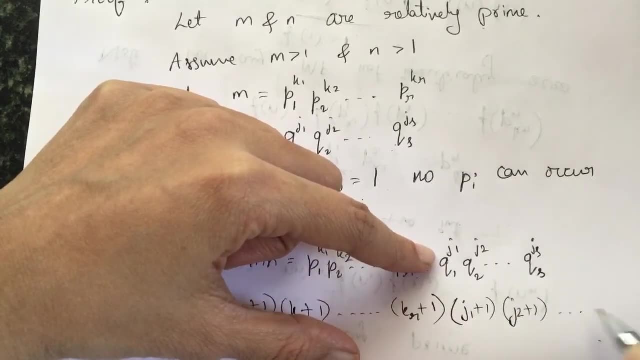 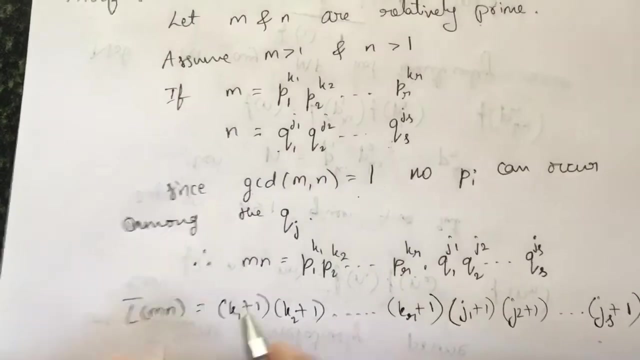 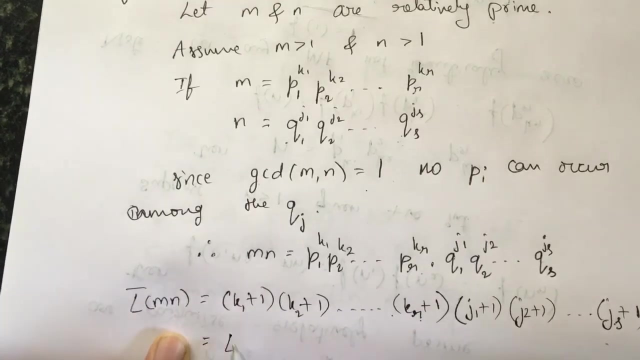 plus 1.. This is for till here. then afterwards powers Jis J1 plus 1, J2 plus 1 up to Js plus 1.. Got the point Now? this is same as writing: K1 plus 1, K2 plus 1 up to Kr plus 1 is nothing but tau of. 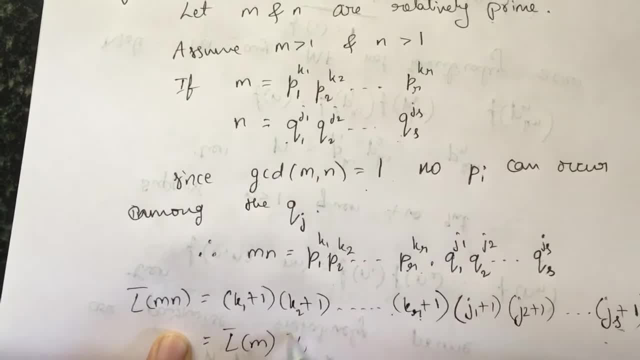 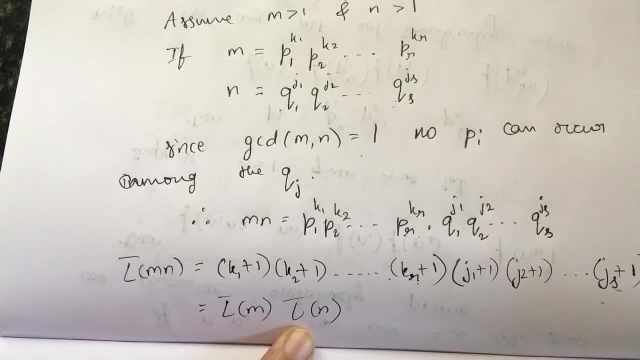 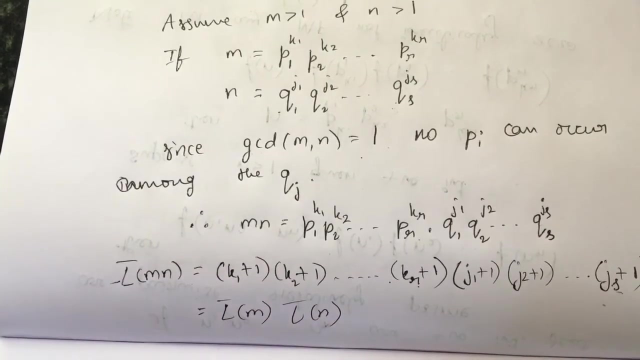 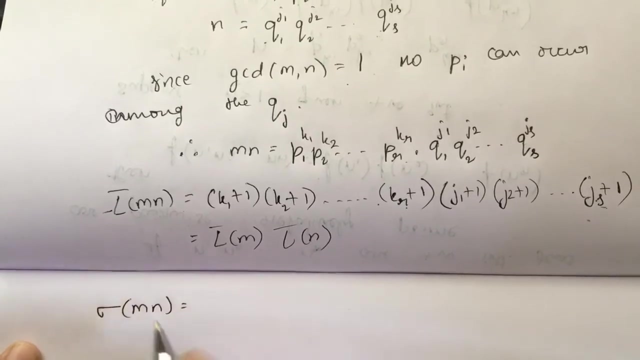 M and this is nothing but tau of Mn, N. Therefore, tau of Mn equal to tau of M into tau of N. So we can say: this is tau is multiplicative function. Now let us look at sigma function. Sigma Mn equal to. we know. 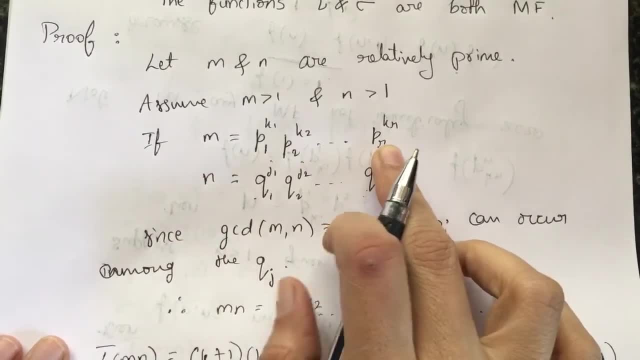 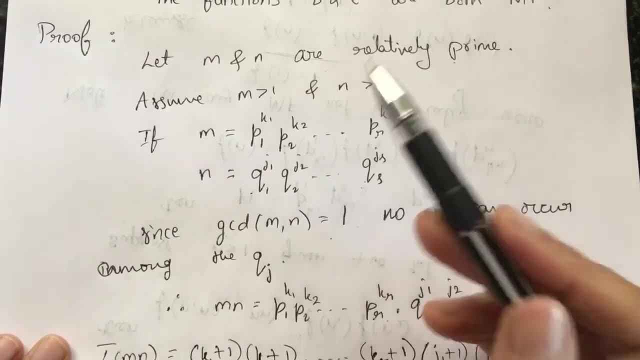 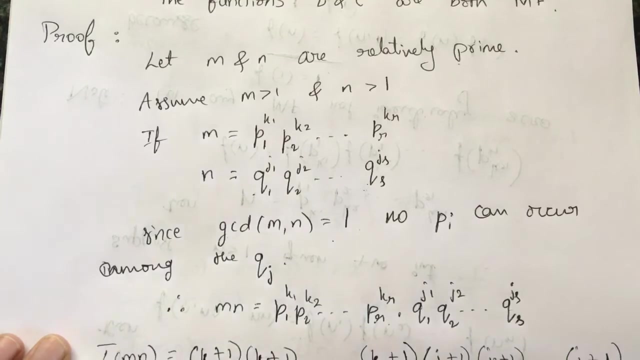 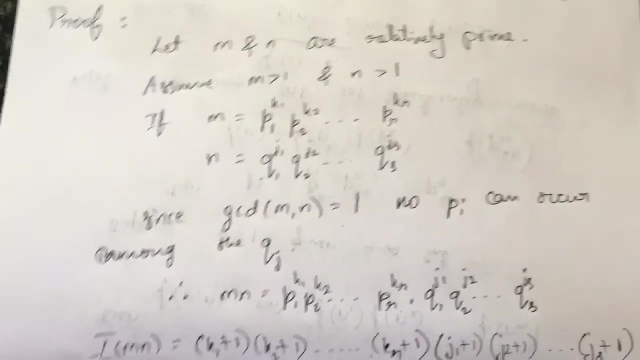 the formula: if M is written like this as a product of primes, then sigma M equal to P1 power K1 plus 1 minus 1 divided by P1 minus 1, into dash, dash, dash, dash, up to Pr power Kr plus 1 divided by Pr minus 1.. I hope you remember that formula. I have mentioned it in my previous video. 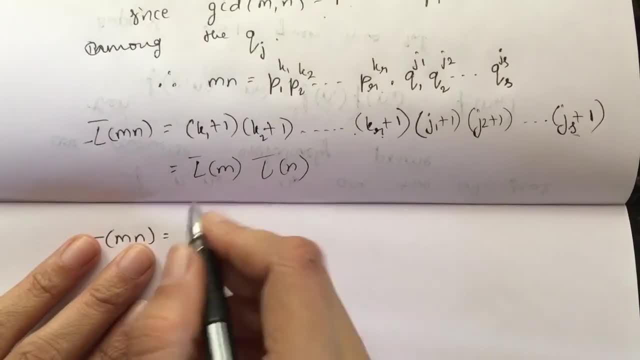 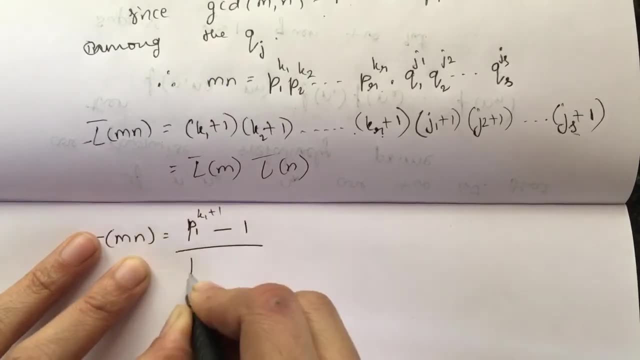 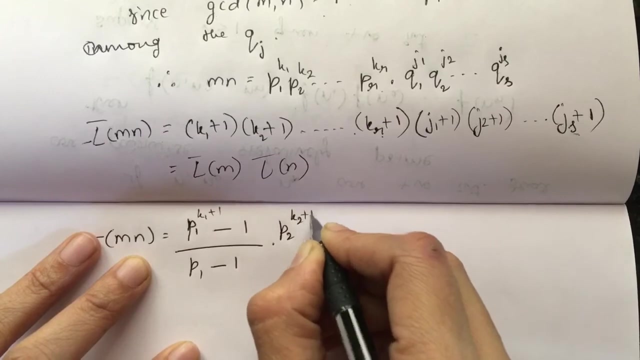 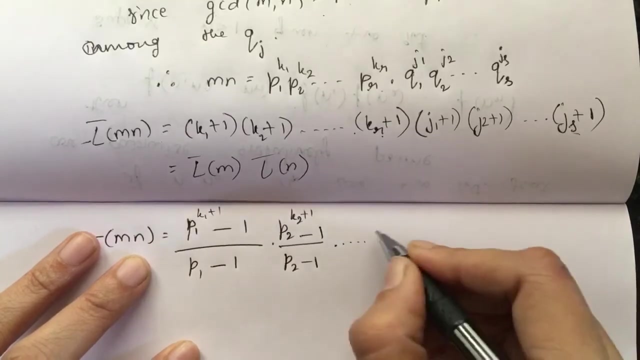 So I will just directly write the values: P1 power K1 plus 1 minus 1 divided by P1 minus 1.. Into P2 power K2 plus 1 minus 1 divided by P2 minus 1. like that: into Pr power Kr plus 1 minus 1 divided by Pr minus 1.. 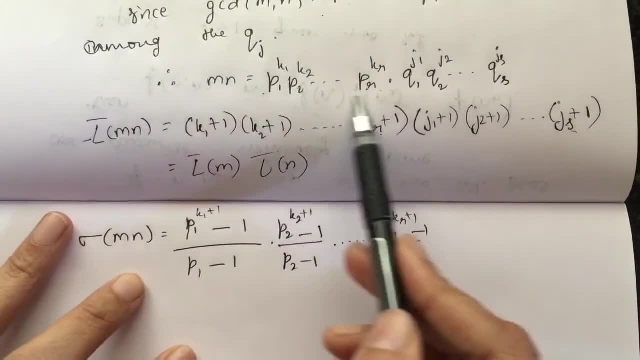 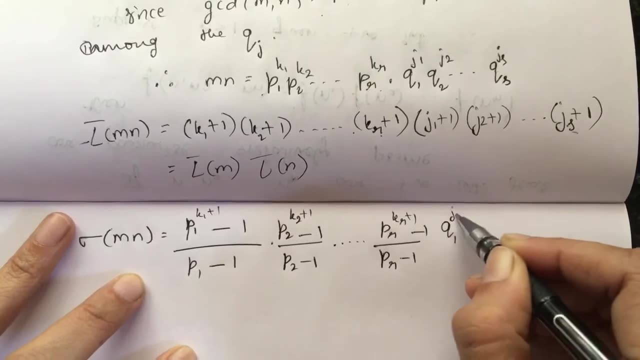 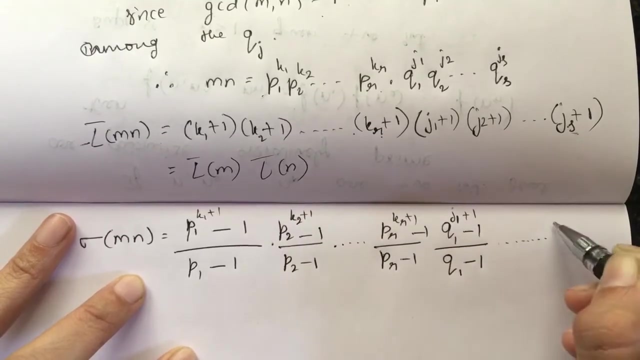 This is for this. much Now for this I have to write it: Q1 power J A1 plus 1 minus 1, divided by Q1 minus 1, into dash dash dash Qs power Js plus 1 minus 1 divided by Qs minus 1.. 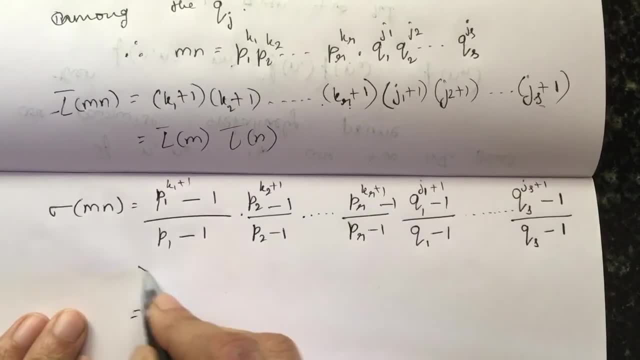 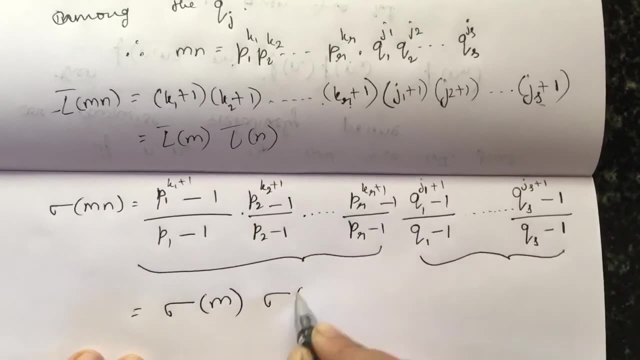 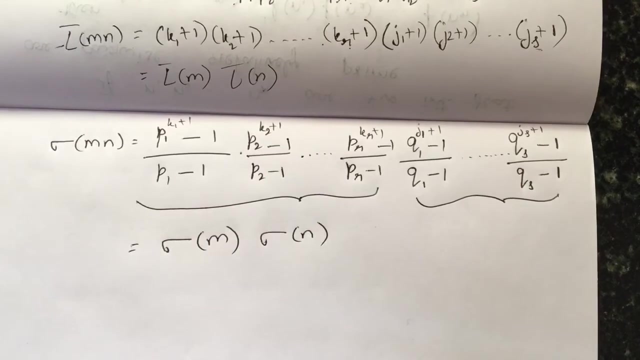 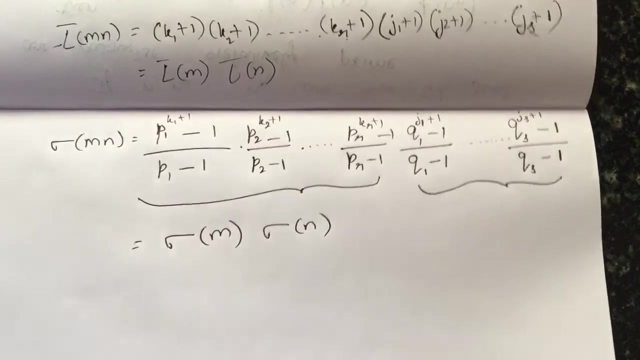 Okay. So when you look at this, this first part is nothing but sigma of M and the second part is nothing but sigma of N. Therefore sigma M- N is equal to sigma M into sigma N. So you can say that the function tau and sigma are multiplicative function, provided the choice of M and N. 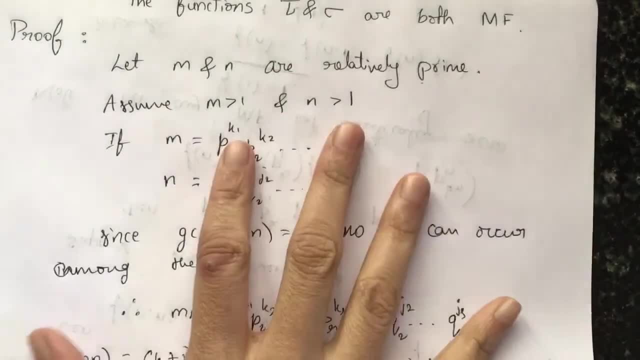 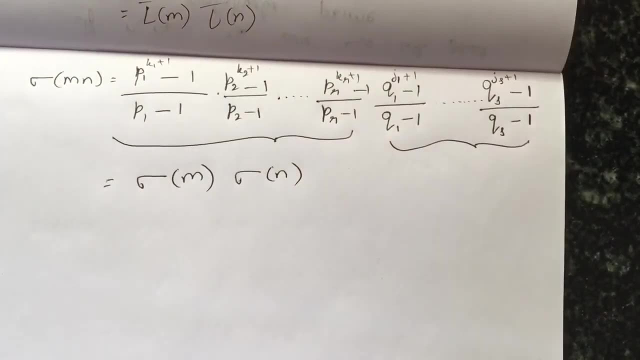 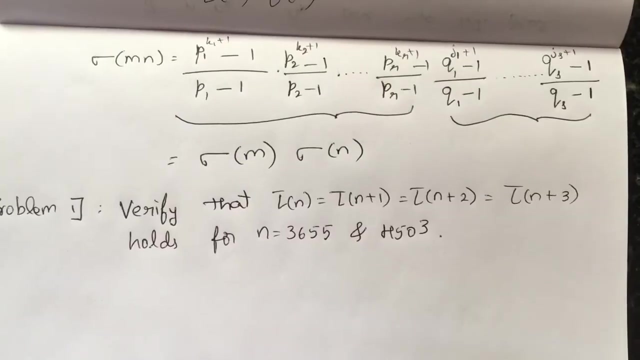 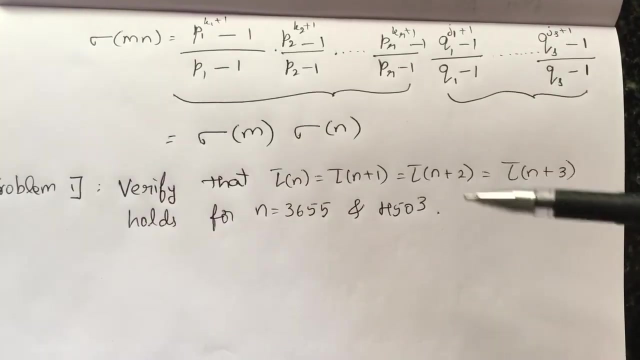 They have to be relatively prime. Then only you can say that the function tau and sigma are multiplicative functions. So just take out one problem: Verify that tau of N, equal to tau of N plus 1, equal to tau of N plus 2, equal to tau of N plus 3, holds for N equal to 3,655 and 4,503.. 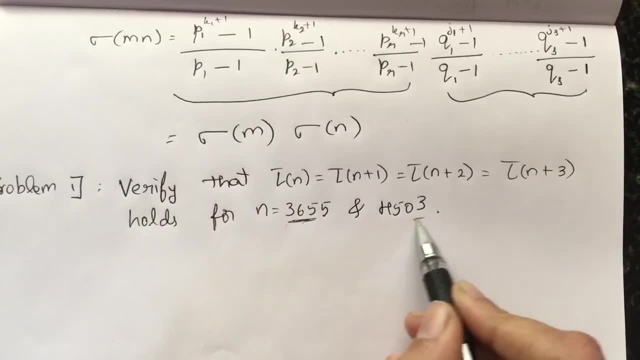 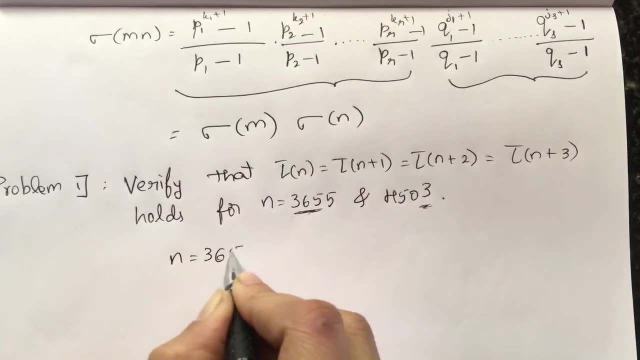 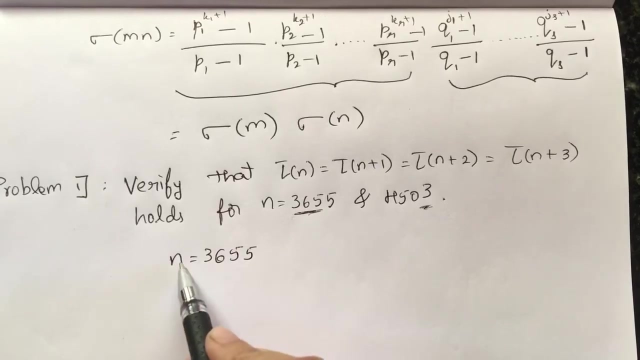 I will just take up this one. You try by yourself this one. Okay, So I am taking N equal to 3,655.. First thing, what we have to do is we have to write the canonical form of N, In the sense I have to write this number in terms of product of primes. 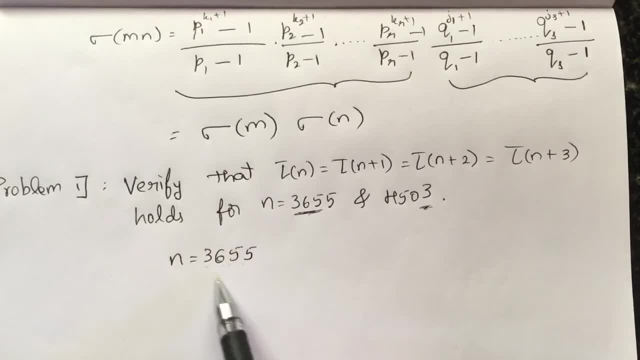 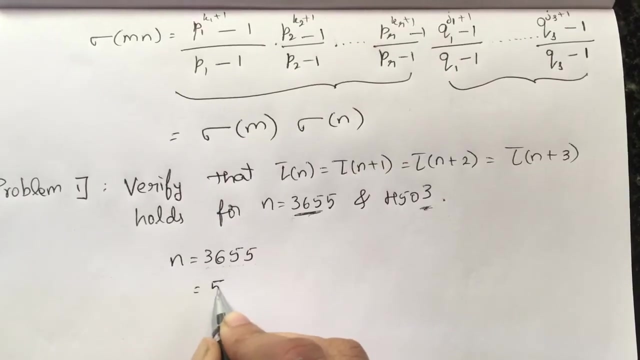 Okay, Since it's 5, always go for dividing by 5 or try to write this in terms of products of 5, because the last digit is 5 over here, So I will just try Write it. Can write it as 5 into 731.. 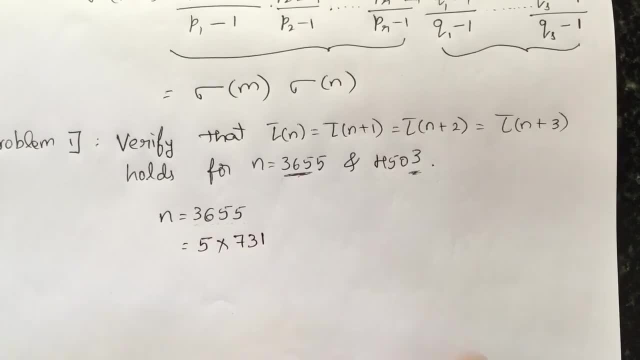 I have already done the calculation, I will just write it down. Okay, So now 731. again, I will try to write it as product of primes, Since its last digit is 1, you try to divide it by 7,, 17, like that. 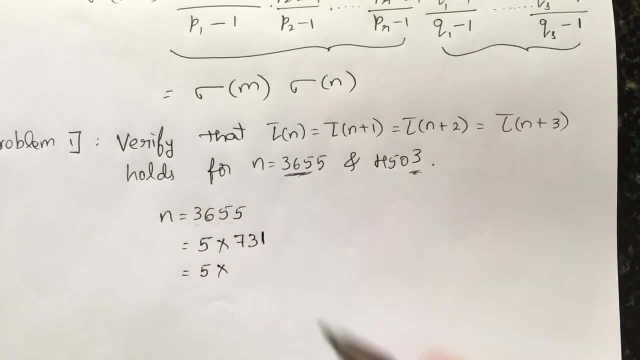 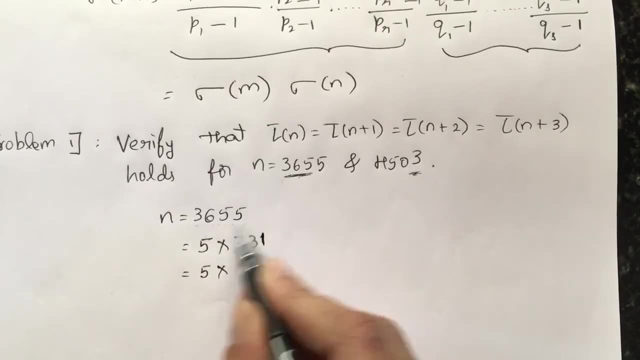 Or 3,, 13, or divide by 9 and all you check it out. Okay, With which number it is completely divisible. Okay, So it can be written as 17 into 43.. Okay, Now it's written in terms of products, of primes. 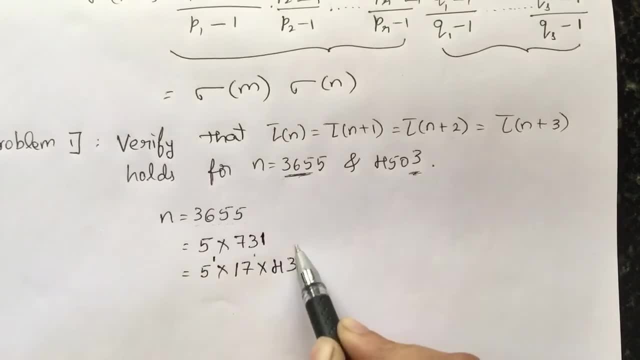 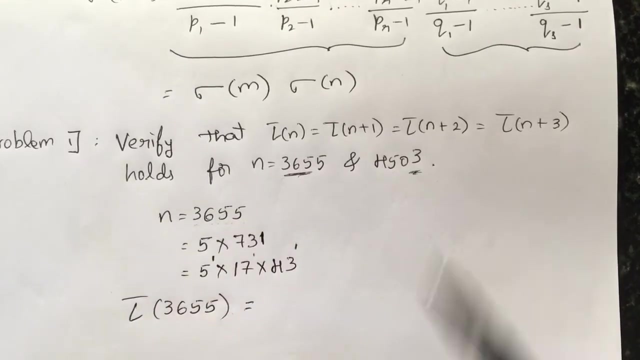 So the powers are 1, 1, 1.. Right, So we will calculate tau of 3,655.. It's nothing but 1 plus 1.. You can use any of the formulas. Okay, You can rewrite this as tau of 5, into tau of 17, into tau of 43. 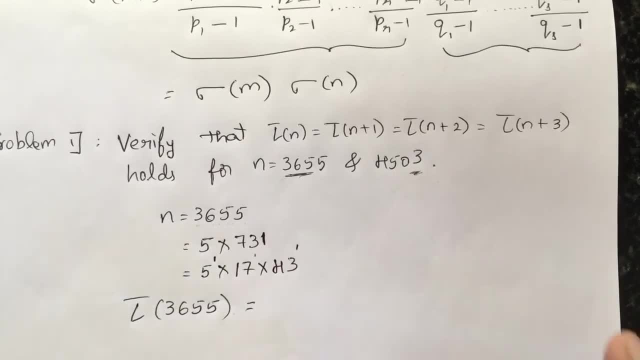 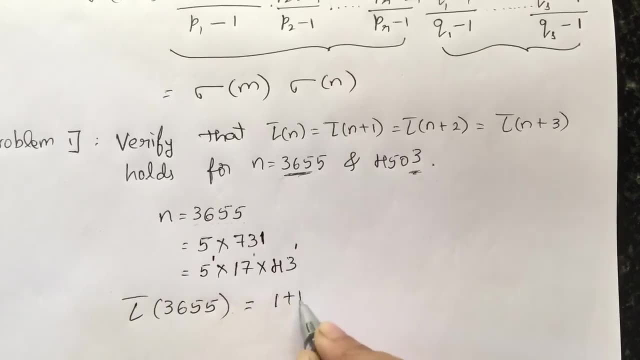 Like that also. you can write, Or you simply take out this powers and write it down. This is 1 plus 1.. This is again 1 plus 1 into 1 plus 1. So it comes out to be 2 cube, which is nothing but 8.. 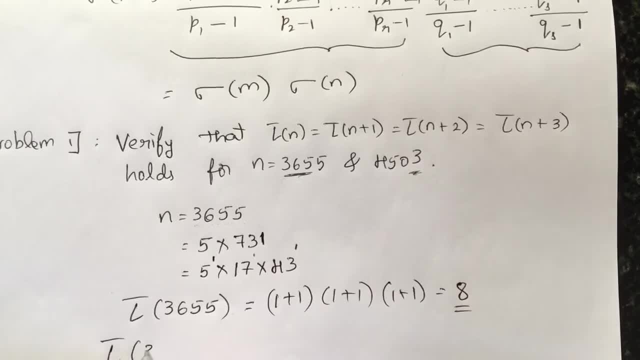 Okay, You can either write it like this: This is the other way of writing This. you can, since it's written in terms of products of primes. You can just write it like this: Tau of 5 into sorry, tau of 17, into tau of 43.. 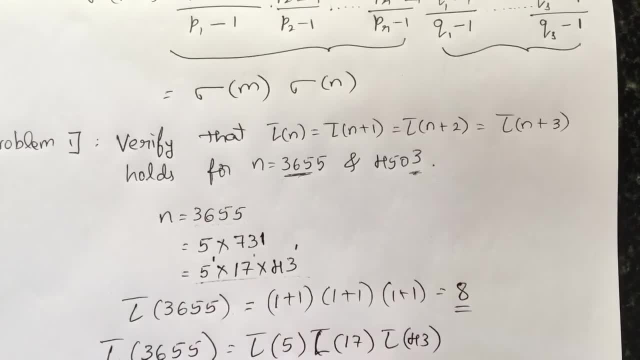 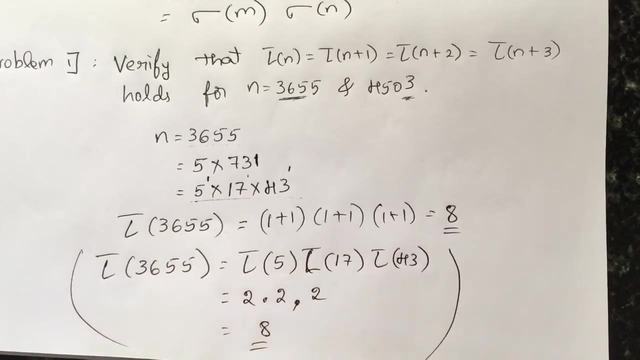 Okay, Tau of 5.. It's 2.. And this is also 2.. This is also 2.. So 2 into 2, into 2, which is equal to 8.. I'm so sorry. Yeah, This way also you can write, or you can just use the formula and do it. 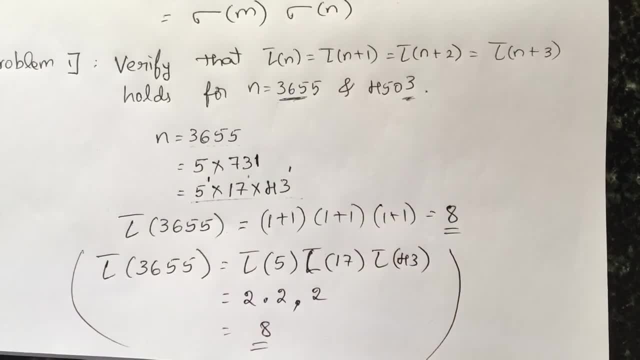 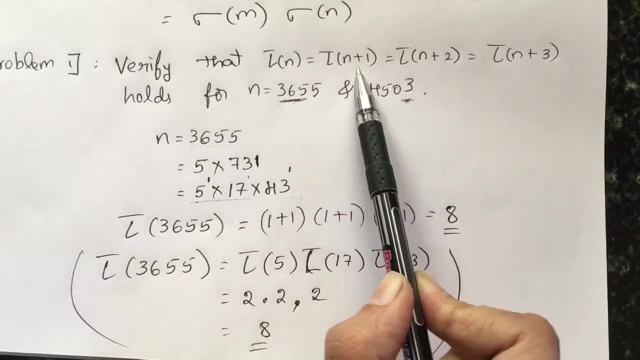 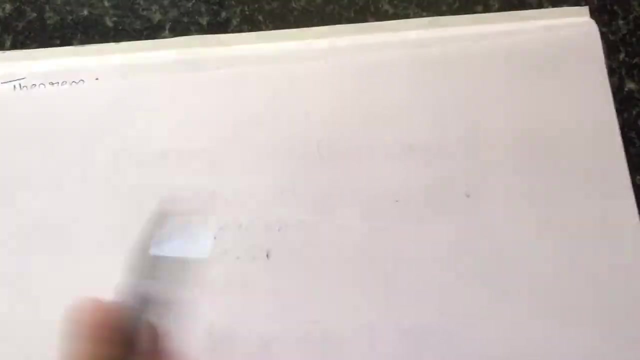 So tau value is 8.. That we got. Now what we have to do. We have to verify tau of n equal to tau of n plus 1.. n is this. I just have to take n plus 1.. n plus 1 is 3, 6,, 5, 6, right. 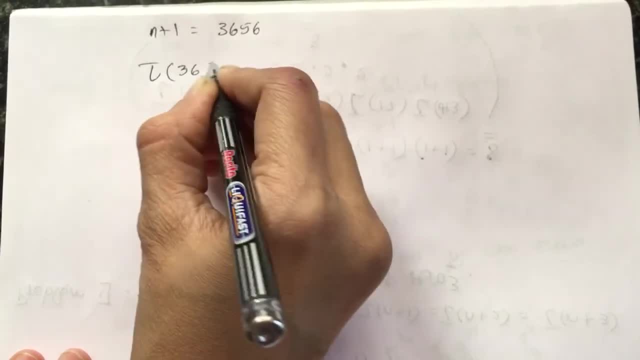 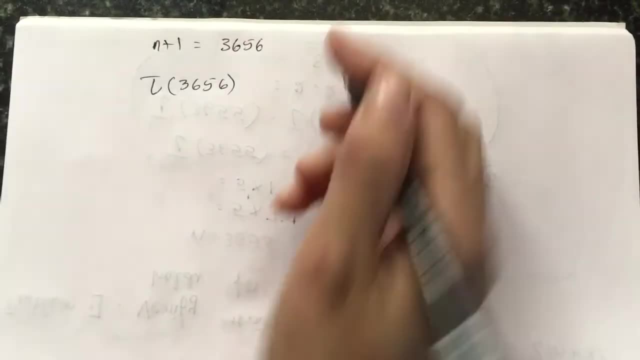 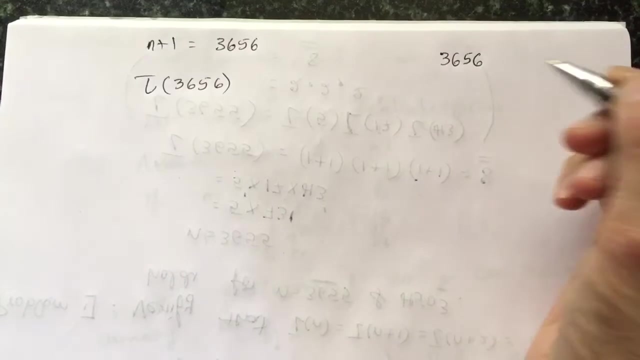 Now I just have to calculate this: 3, 6,, 5, 6, for that I have to rewrite this number in terms of products, of primes, Say 3, 6,, 5, 6.. Hmm, Uh. 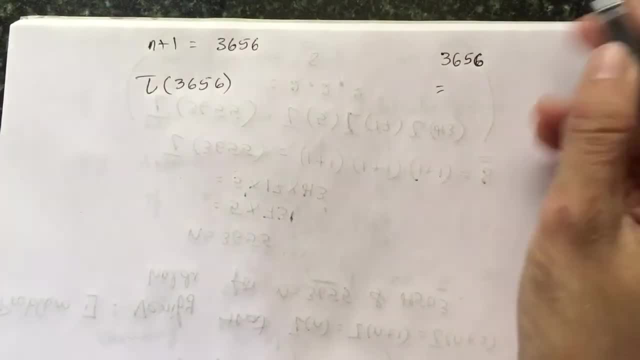 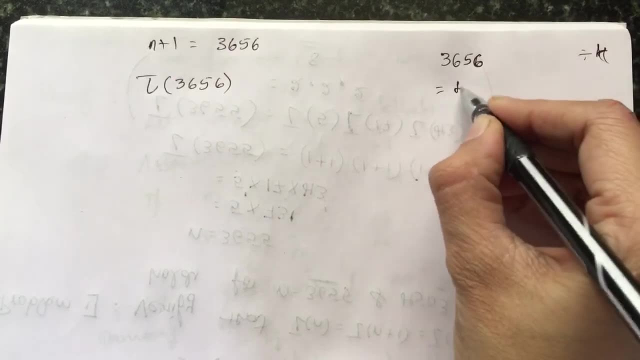 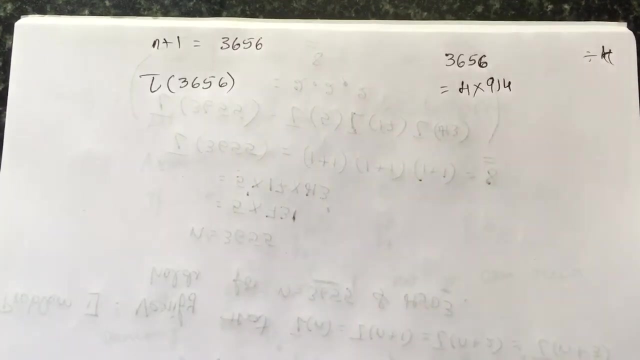 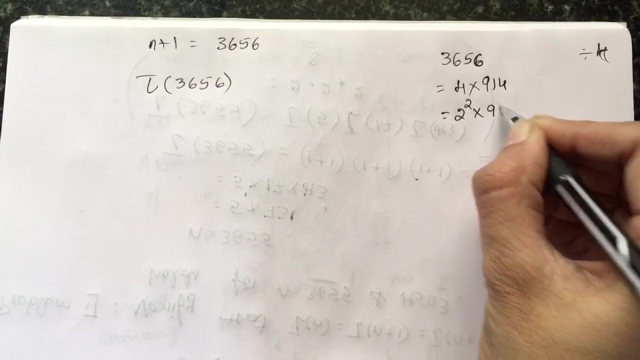 Can be written as: since it's ending with 6.. Let me divide it by 4 first. Hmm, Uh, I'll write it in terms of products of 4.. Product of 4.. Yeah, Uh, 4 can be written as 2 square into 9, 14.. 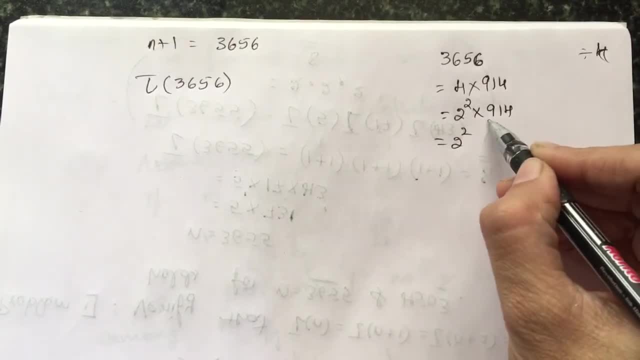 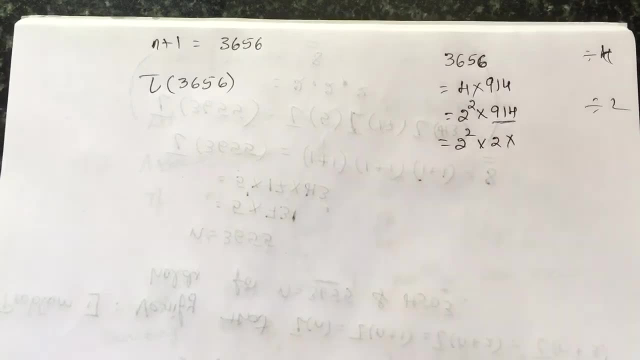 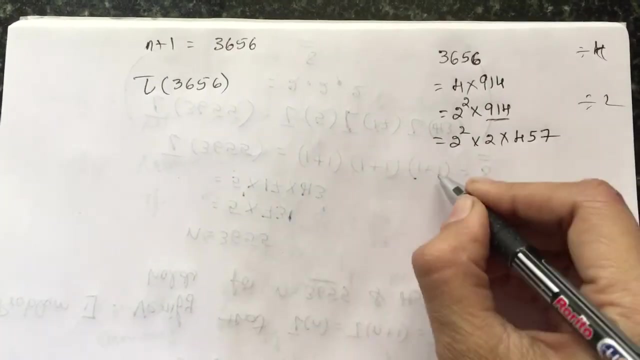 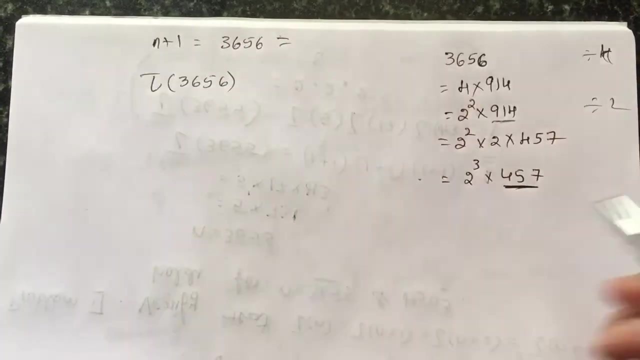 Now this 14.. Uh, Again, I can, I can divide it by 2, I guess. Yeah, So that it's 457.. Yeah, Now you can observe one thing: This is a prime number. Hmm, So it's written in terms of products, of primes. 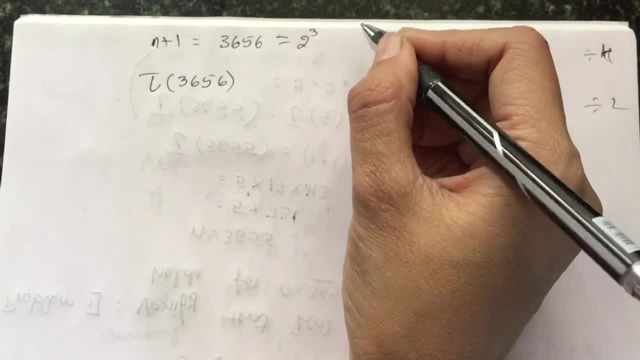 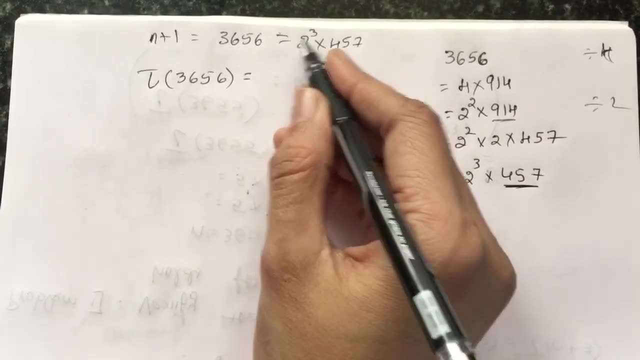 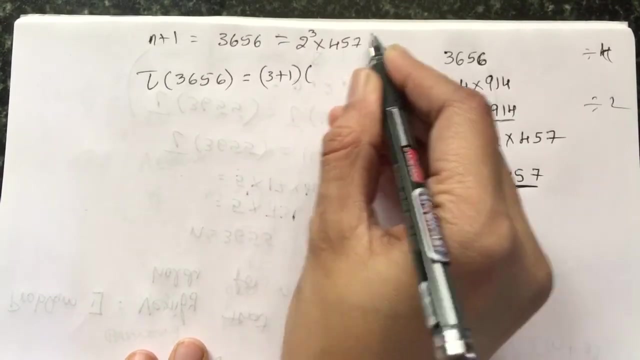 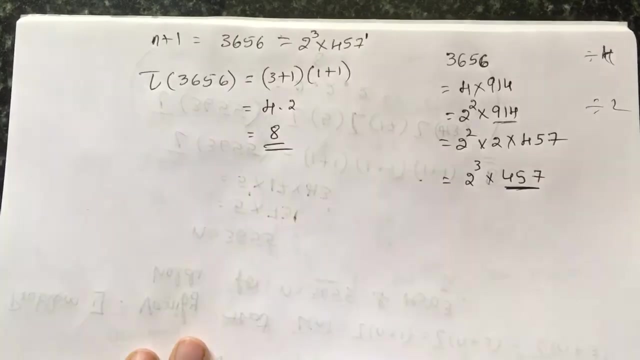 Now 2 power 3 into 457.. So this is power 3, 3 plus 1 into power 1, so 1 plus 1, so it's 4 into 2, again 8.. So 2 of n plus 1 is also 8.. 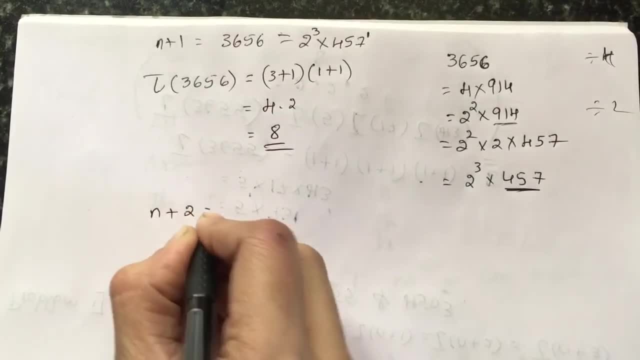 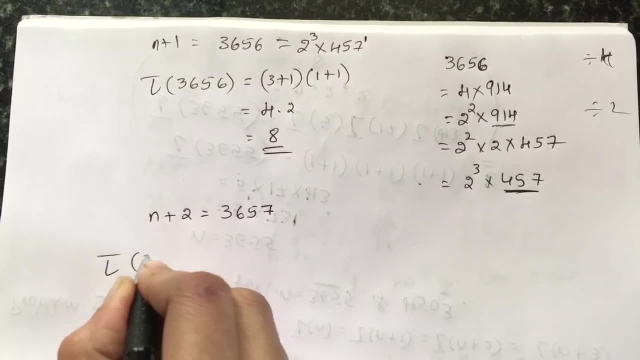 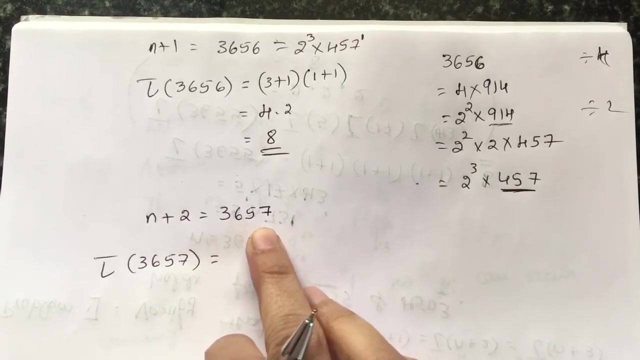 Now we'll take n plus 2, it's 3,, 6,, 5,, 7.. Hmm, So I have to calculate 2 of this number. So since it's ending with 7, I'll just divide it by 3 first. 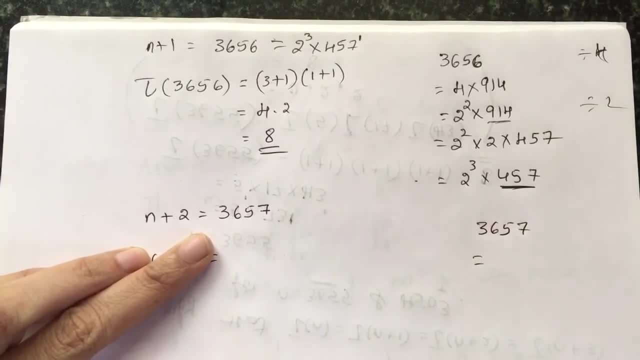 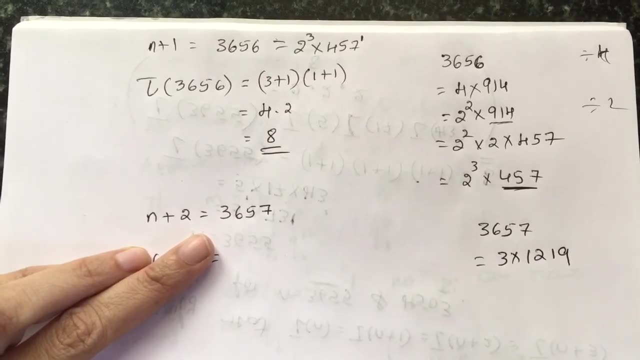 Hmm, So it's 3 into 1, 2, 1, 9.. Then again, this is ending with 9.. So 3 into 1, 2, 1, 9.. Then again, this is ending with 9.. 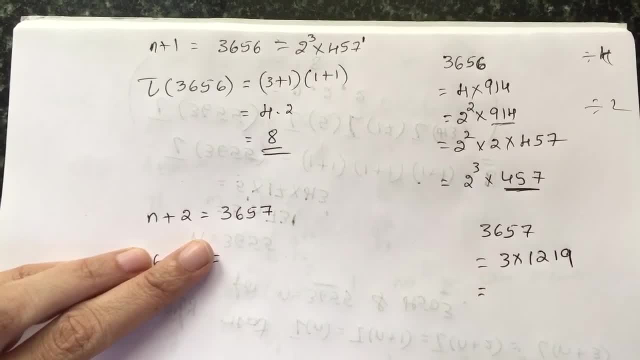 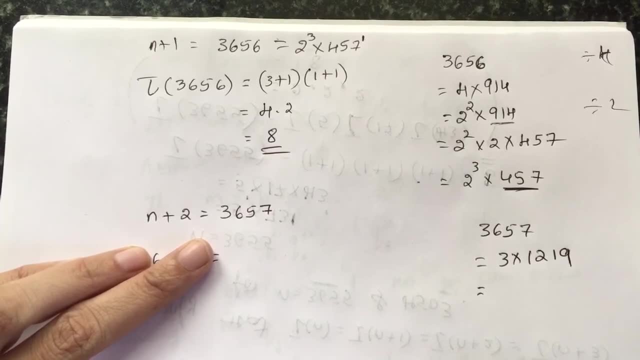 So 3 into 1, 2, 1, 9.. So 3 into 1, 2, 1, 9.. So this should be a multiple of 9 or 3.. Hmm, Okay, okay. 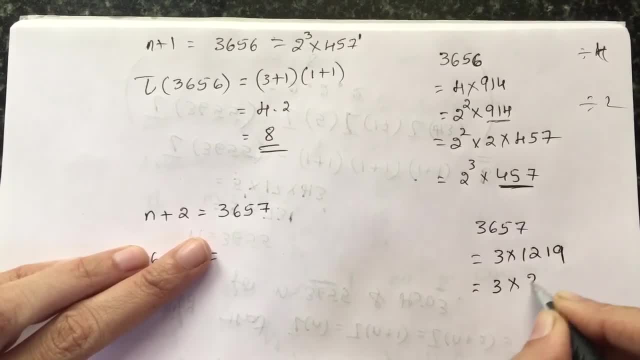 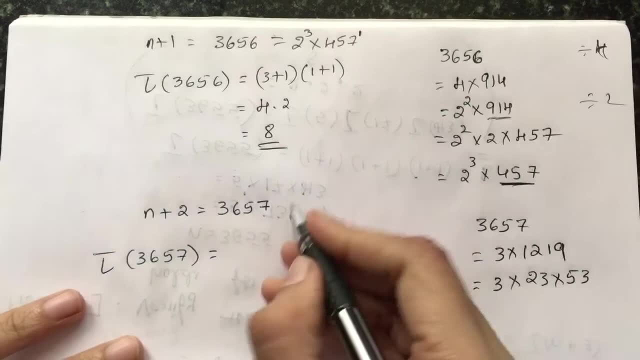 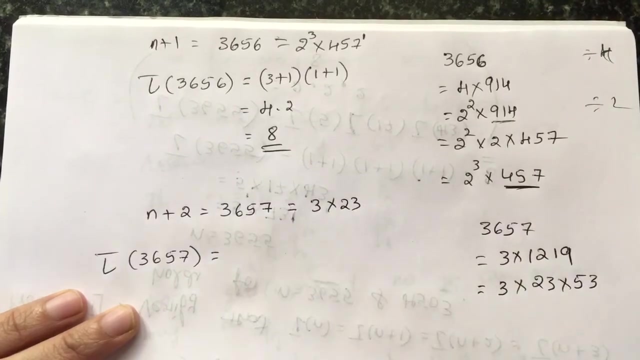 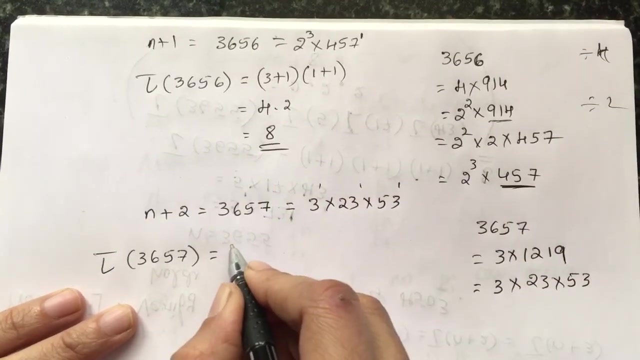 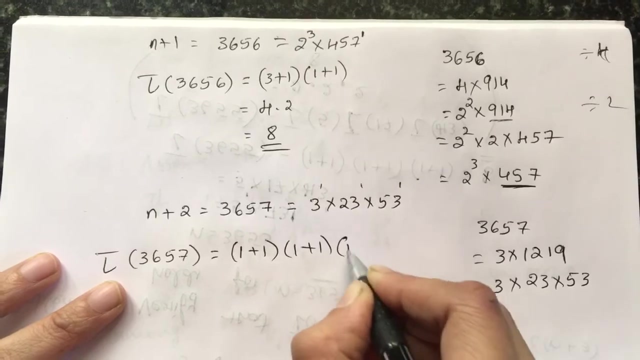 Yeah, Can be written as 23 into 53.. Yeah, So I'll just rewrite this as 3 into 23.. 1 into 53. again, these two are prime, so powers are 1, so can directly write 2 of 3, 6, 5, 7, 1 plus 1 into 1 plus 1 into 1 plus 1, so it's 2 power 3, which is equal to 8, so you. 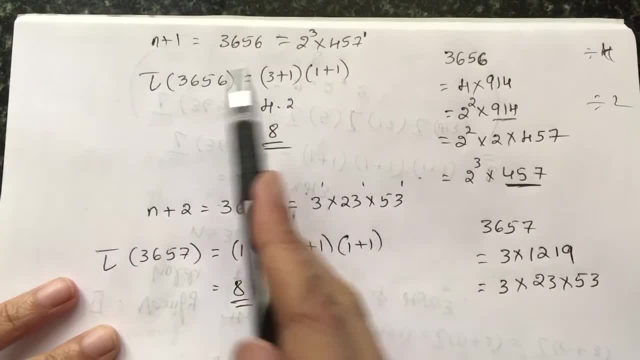 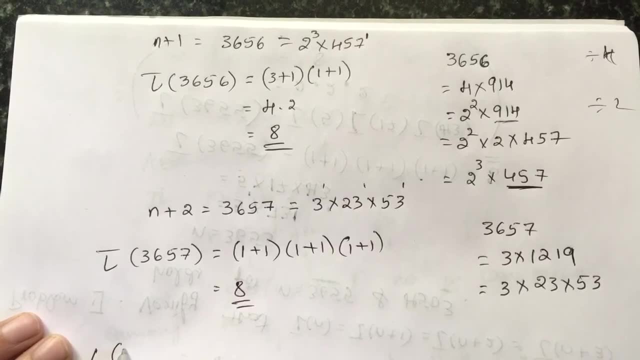 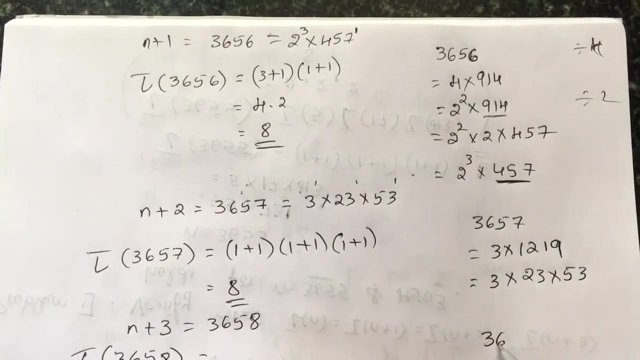 observe one more thing: 2 of n, equal to 2 of n plus 1, which is equal to 2 of n plus 2. the last possibility is 2 of n plus 3. it's 3, 6, 5, 8. 2 of 3, 6, 5, 8. 3, 6, 5, 8 can be written as: 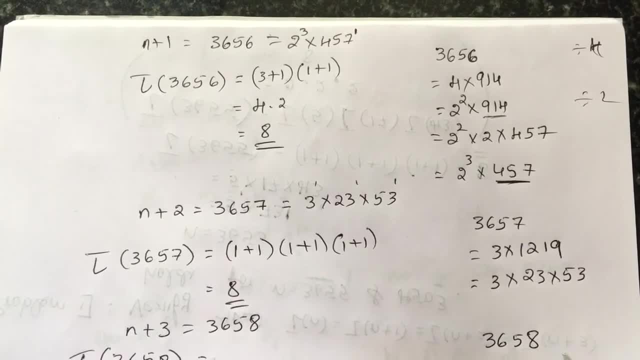 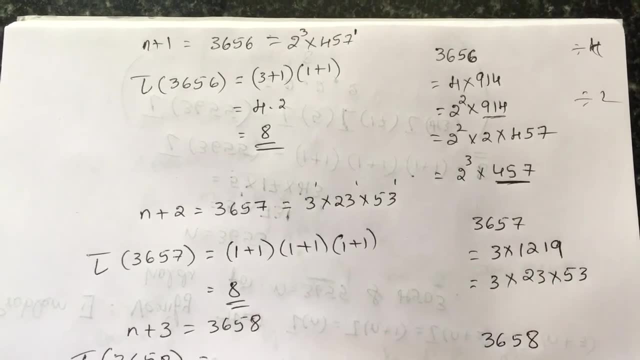 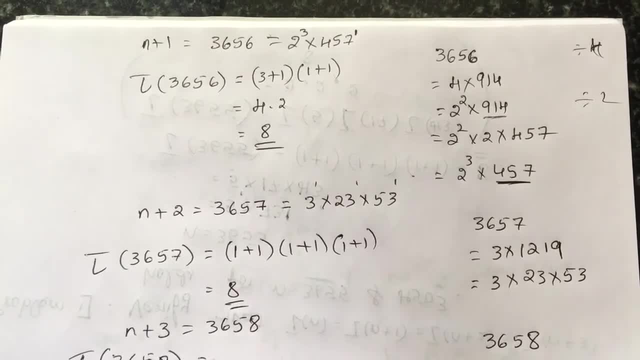 we go by dividing it by 2. that could be easier. 1829, since it's 9 over here, we easier. 1829, since it's 9 over here, we easier. 1829, since it's 9 over here. we divide it by 3 and check. 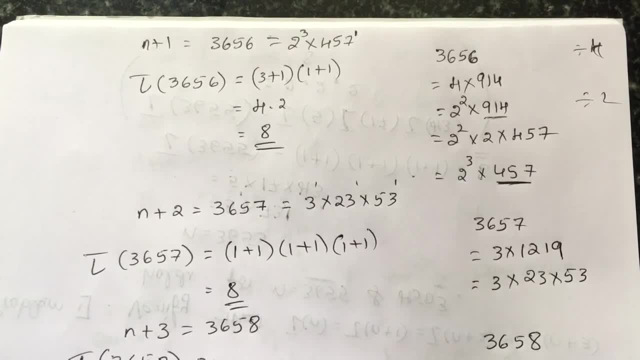 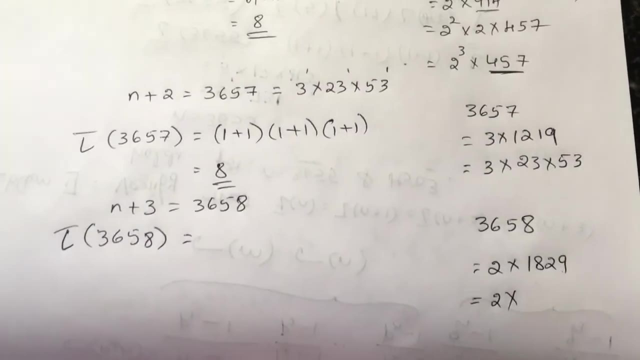 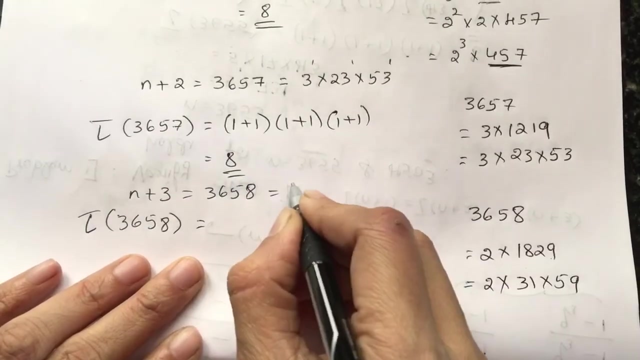 divide it by 3 and check. divide it by 3 and check: okay, this can. okay. this can be written as: sorry. this can be written as: 2 into 31 into 59, so it's 2 into 31 into 59, so it's. 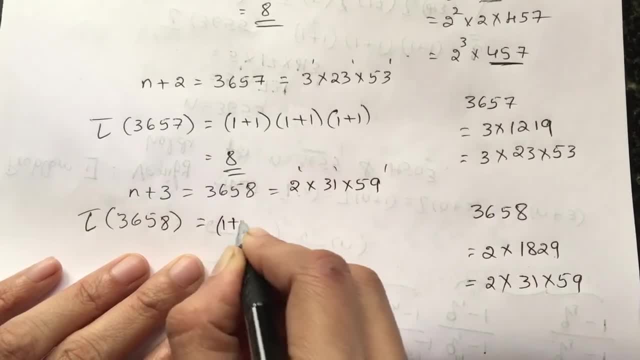 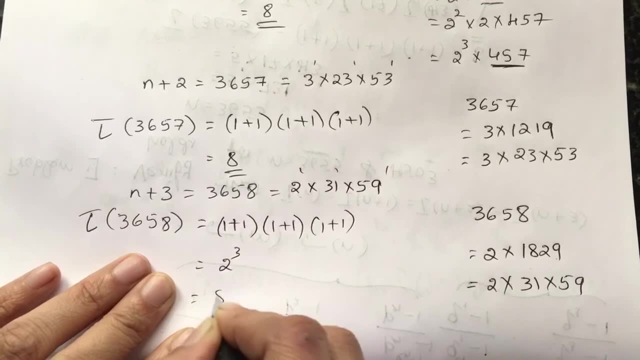 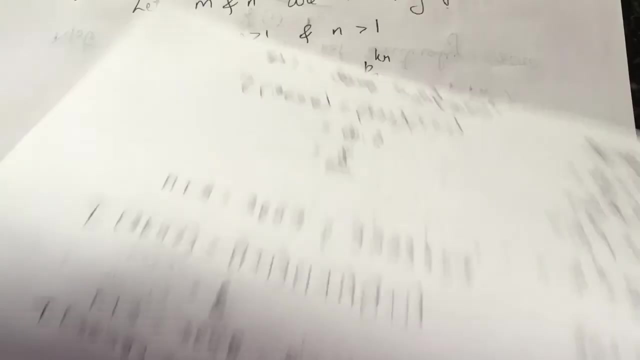 again, the powers are 1, so 1 plus 1 plus 1 into 1 plus 1. i'm directly using the formula, so 2 cube, which is nothing but 8. so verification is done over here for n equal to three, six, double five.